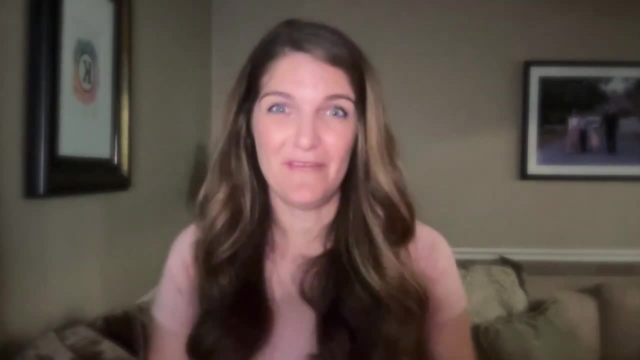 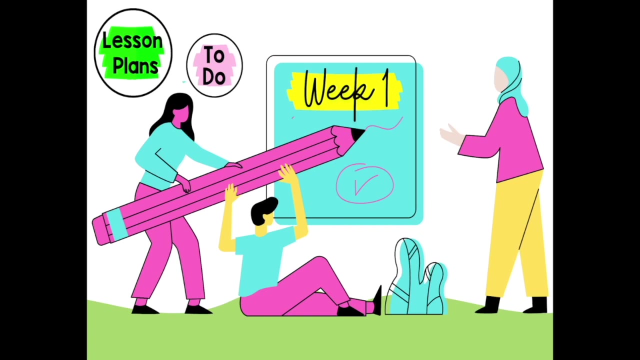 So here is what I do the first week, So let's check it out. This is the planning guide to go with the first week and let's check it out. I have it broke down between lesson plans and then to do things like things you need to do to prepare for the week. 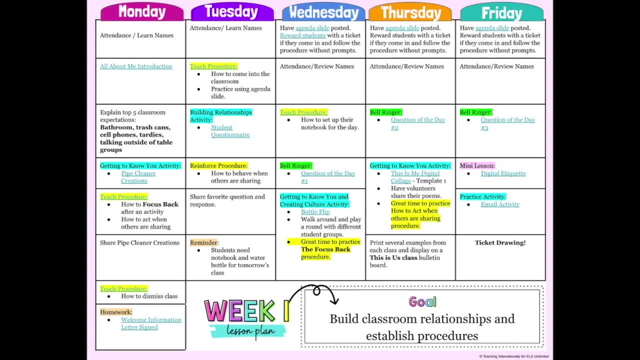 So it looks overwhelming, but let's take it step by step. Let's go to Monday. So Monday, what you're going to do is, very first thing is you learn these Names, because the name is the most important thing for your students, for anybody really. 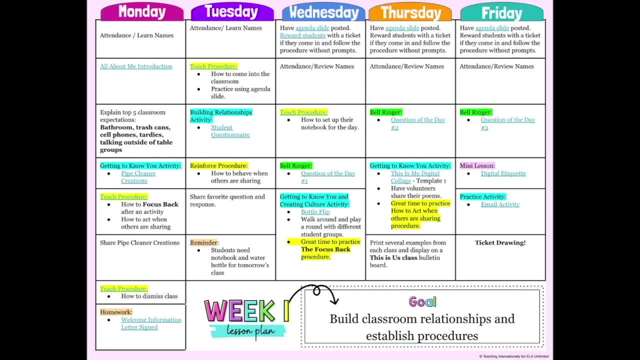 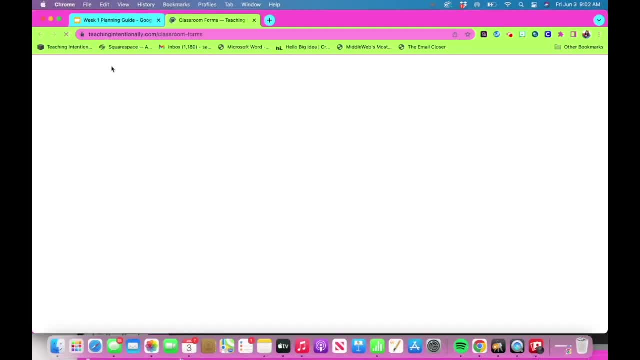 So you really want to value that for them and take time to learn their names. After that, you do it all about me: introduction, And what I like to use is this bit moji right here. So this is what I like to use. 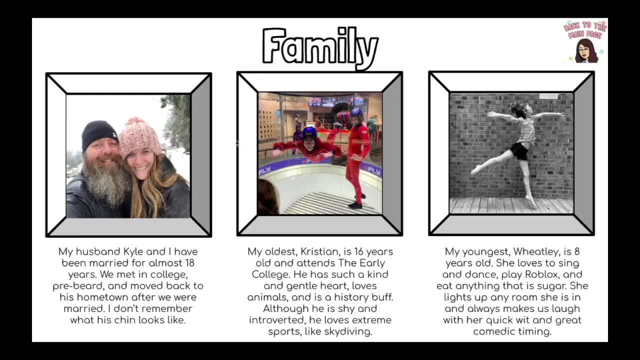 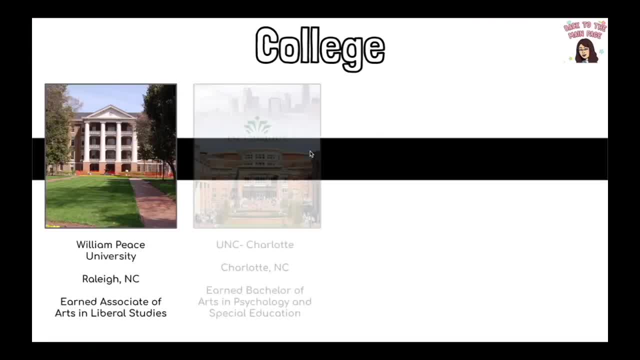 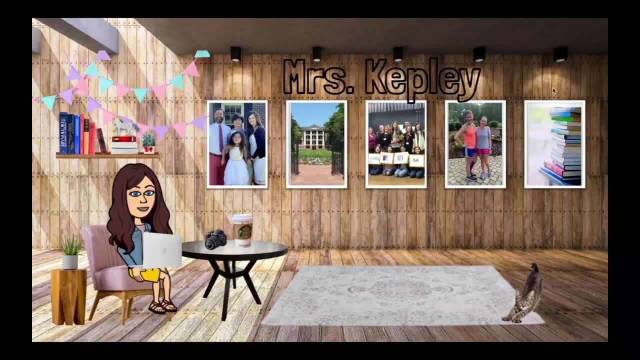 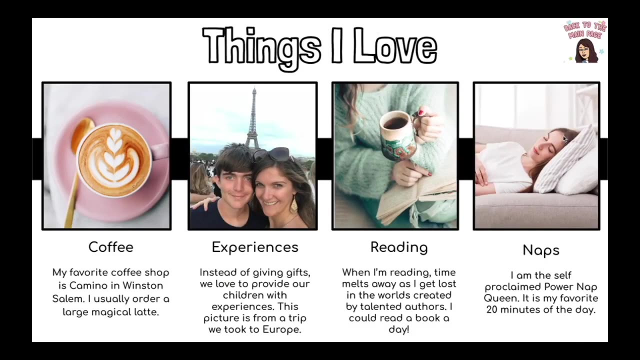 It's a bit moji all about me, where we can just click on the different frames and it tells my students about my family, Where I went to school, My why I love teaching what I do in my free time, and then any supplies that we need for the classroom and things that I love. 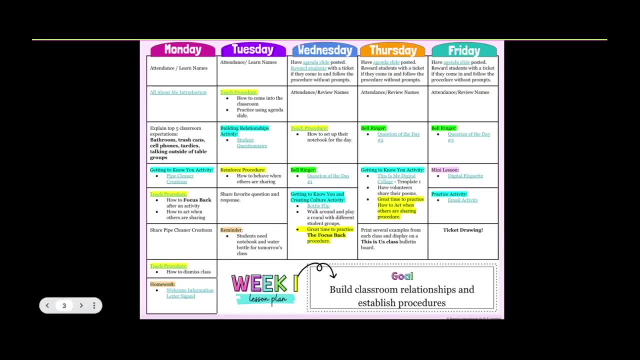 So after we do that, that shows your students that you are a person and that you have things outside of the classroom, and it also will start building connections with your students. After that, I explain my top five classroom expectations, which is how to get to the bathroom. 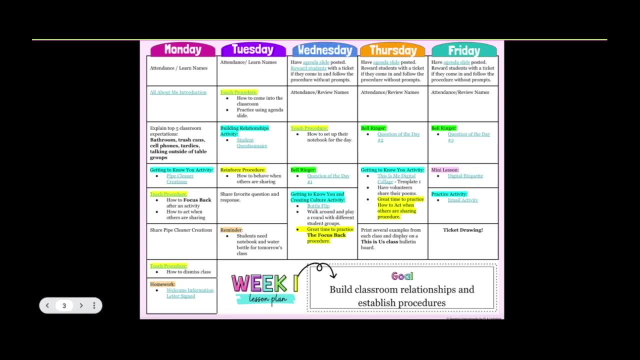 We don't get up and walk to trash cans. We have trash cans on our table. What to do with cell phones, my tardy policy and what I call talking outside of your table group. So if we're doing collaborative work, talking to a neighbor or at another table, so I go over. 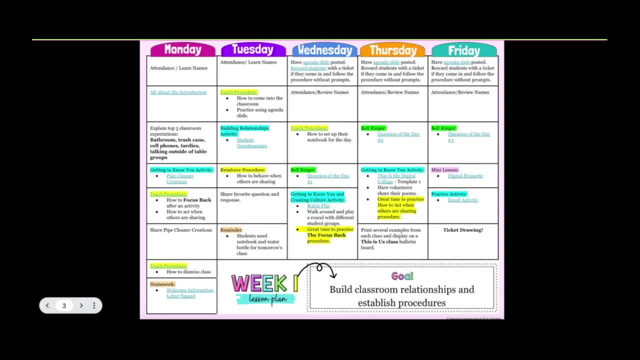 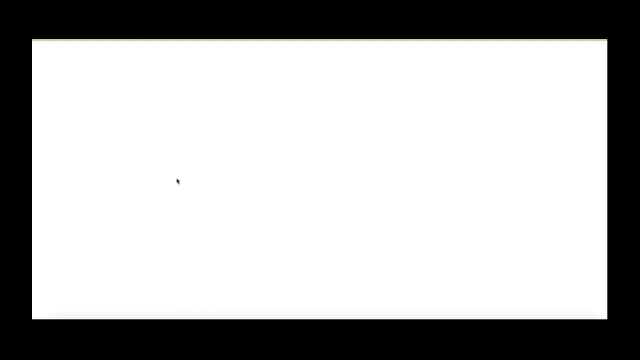 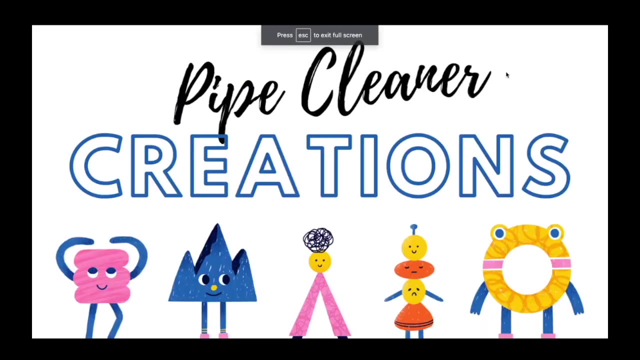 Those are my really big five expectations for the classroom. And then we do. We do this fun getting to know you activity And it's on here. Let me get it for us really quick. So with this activity, I call it pipe cleaner creations. 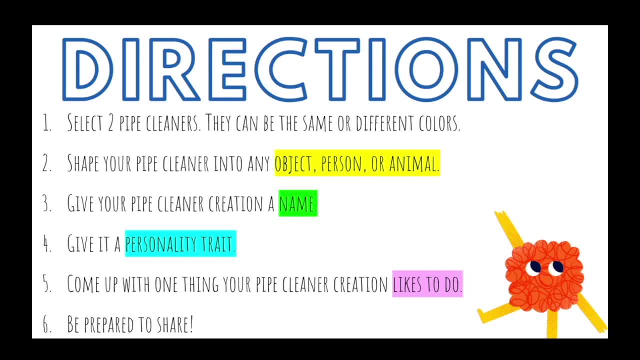 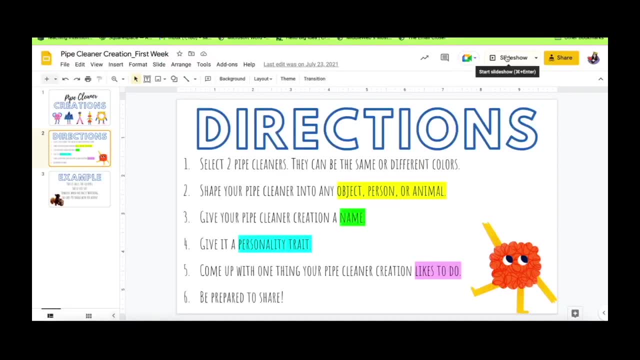 And so each students get pipe cleaners and they shape their pipe cleaner into an object, a person or animal. They give it a name, They get a personality and they come up with something that the creation likes to do, And then they share it with everybody. 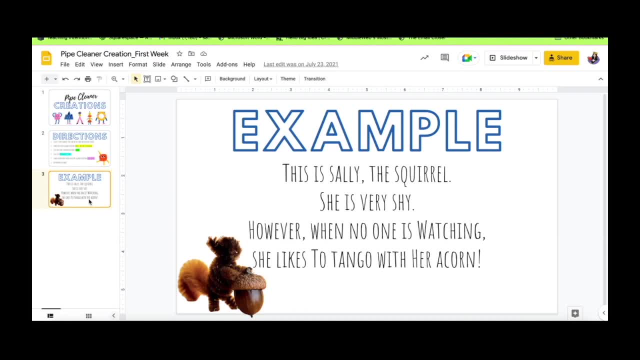 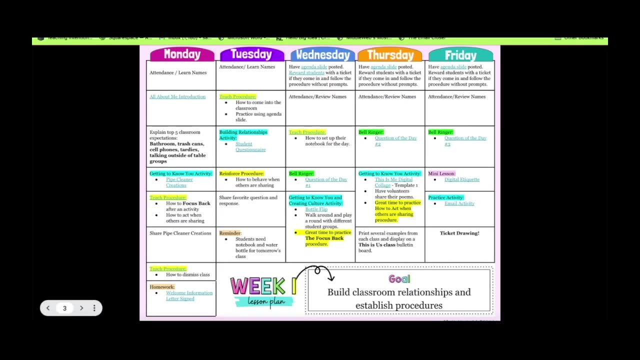 So I always give an example. So this is Sally, this girl. She is very shy. However, when no one's watching, she likes to tango with acorns, So it kind of gets them moving, it doing something with their hands, instead of just sitting in the classroom and sitting at the table and doing something that every other teacher is doing. 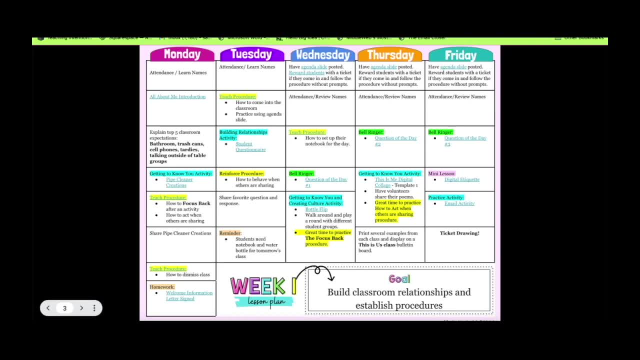 And it's. it's funny, They end up creating really fun things After that. I teach them how to focus back after night. I teach them how to focus back after night. I teach them how to focus back after night. I teach them how to act when others are sharing and then they share their pipe cleaner creation. 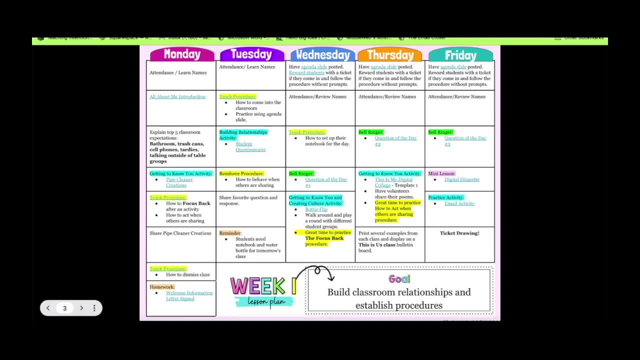 And we practice these procedures of how to focus back and how to act when they're sharing. I make sure I really praise students who are, like, really involved and showing a lot of enthusiasm for the activity. After that I teach them how I dismiss the class, which is no one gets up unless I tell them to. 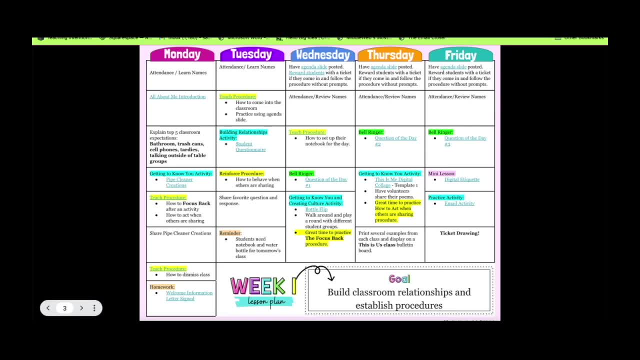 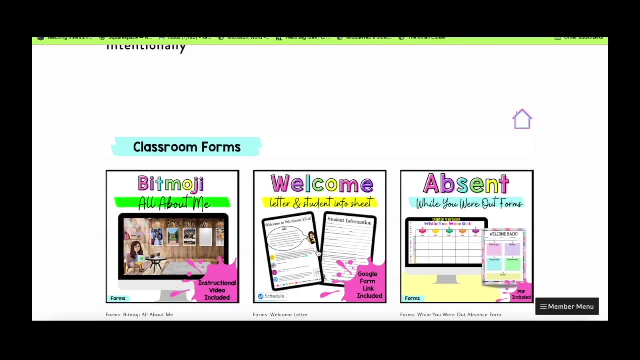 I hate students lining up at the door And I say have a great day And they say hi and they leave. So I do give them a little bit of homework, which is getting an information sheet signed. So it's right here, The Welcome student letter and information sheet. 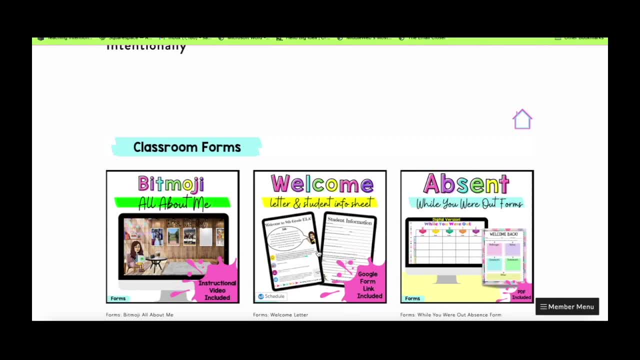 It tells them my Google Classroom code, my Amazon wish list, my Remind code, any important information, And then I get some information from them. So I print one good note as soon as I get that. So I print one color for each class and I pass those out at the beginning. 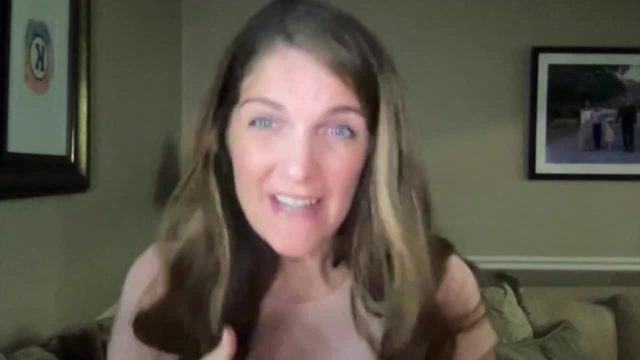 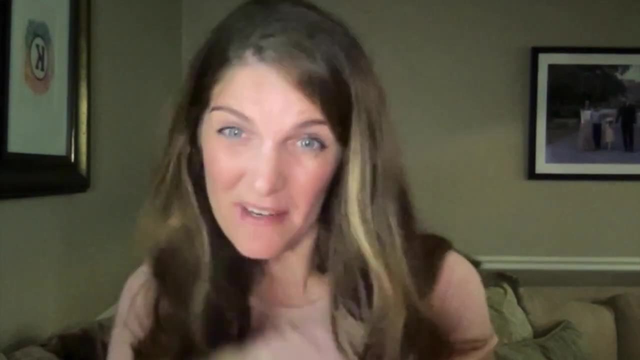 So that's the first day. It kind of really establishes relationships that you're going to have fun in the classroom, but you're also one that has expectations. So we're going to roll into Tuesday. You're going to start the same way. 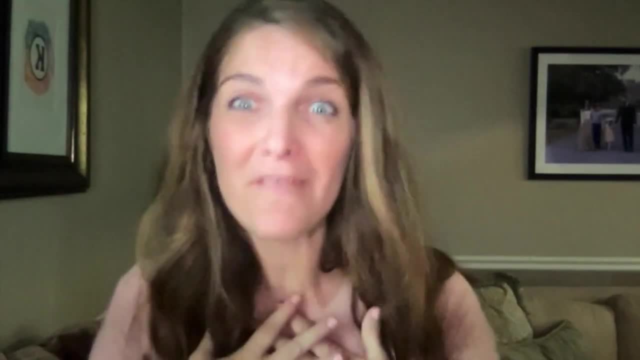 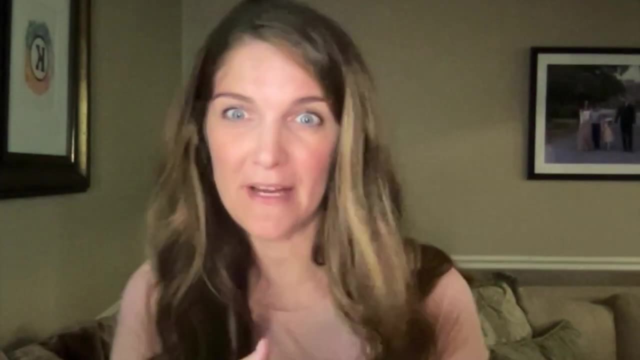 You're going to go over the names, see how many you can remember. A fun way that I like to do it is I have a basket of questions like random questions, like what's your spirit animal? Um, if you could drive to school with one person, who would it be? 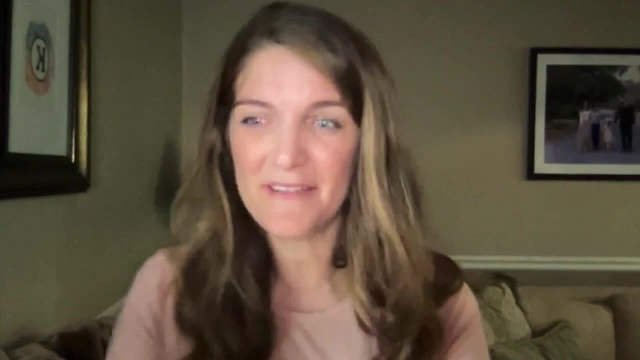 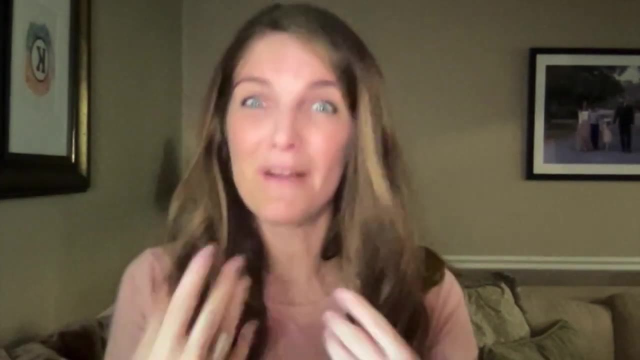 Do you like your Pop-Tarts- warm or cold, Like that kind of stuff? So when I call someone's name, I draw out a question and they answer it. So it helps me start to make connections between names and what they like. 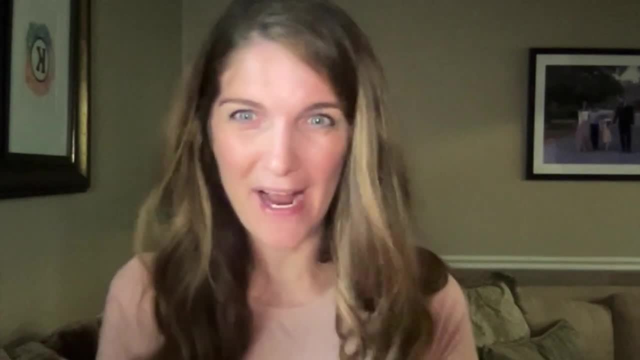 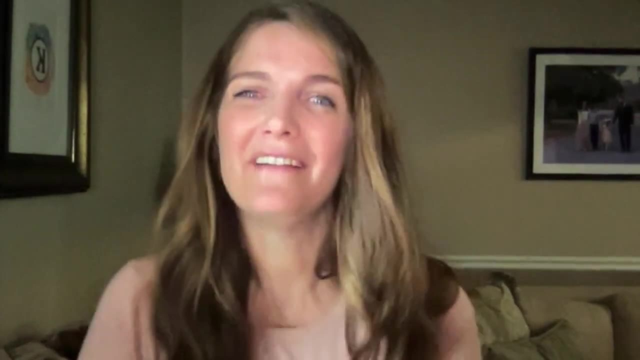 And it like um. one person said they like to eat dry ramen noodles and so, um, I call her Dry Noodle Drew because her name was Drew, Anyway, so that helped me remember. So after we go over, 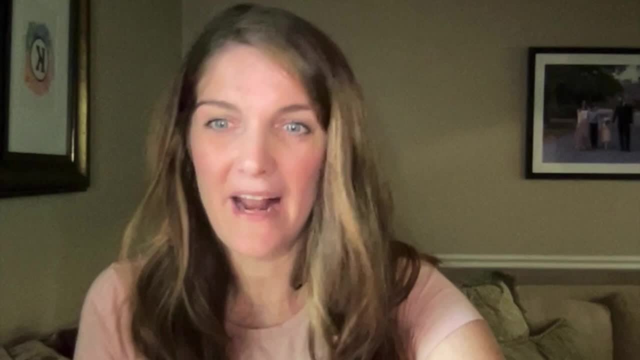 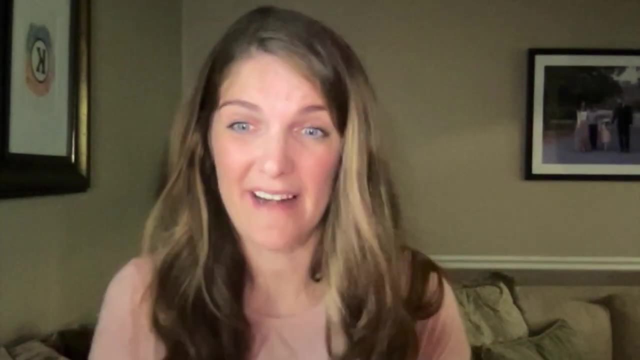 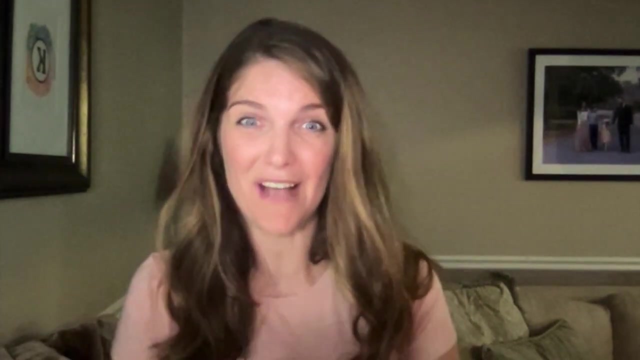 names again on Tuesday. what I do is I really work on establishing my coming into the classroom procedure and getting organized, And so I don't know about you, but I have seen students. when I was a special ed teacher, I co-taught in classrooms. 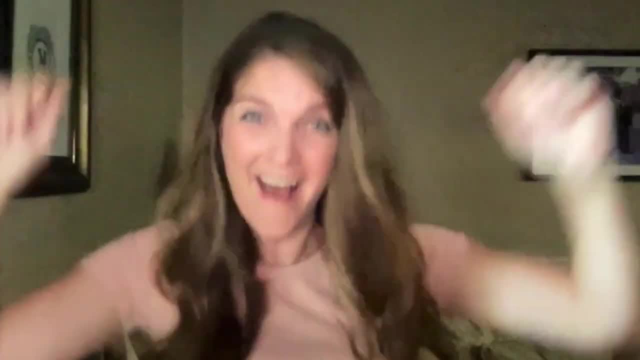 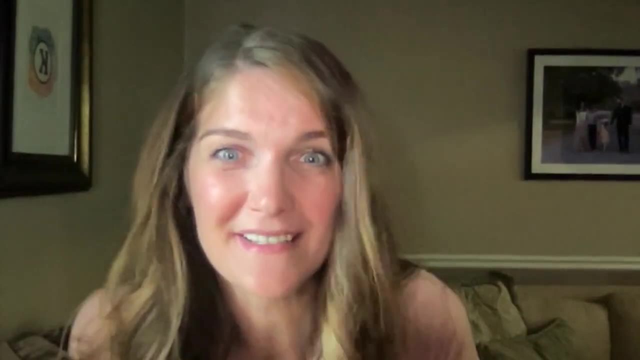 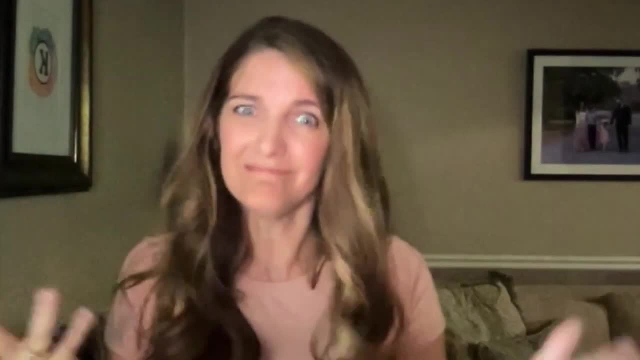 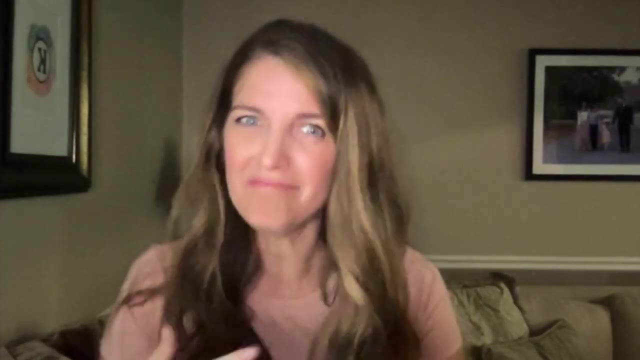 Okay, Okay, Okay, Okay Okay. Like you know, you teach middle school. They're a, they're a little wild sometimes, And so when I have my own classroom, I was like I'm I'm that comfortable with that. 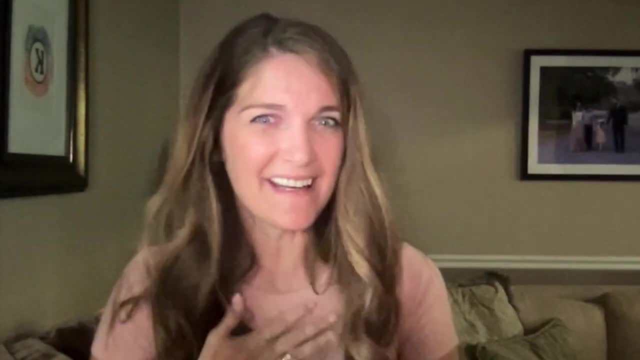 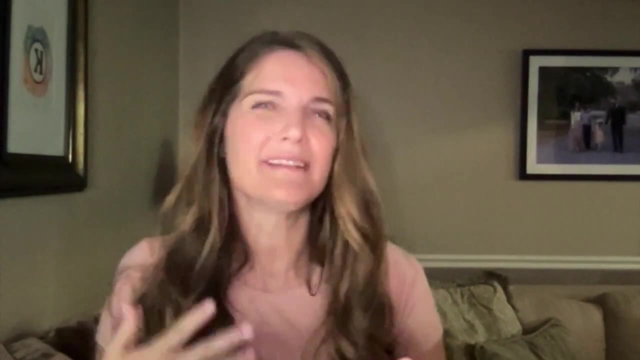 level of them coming into the classroom, Um, and so I needed to come up with a procedure to teach my students how to come into the classroom. And everybody's like they're eighth graders. They should know. Yes, they probably should know, but I can't fault them and get mad at them. 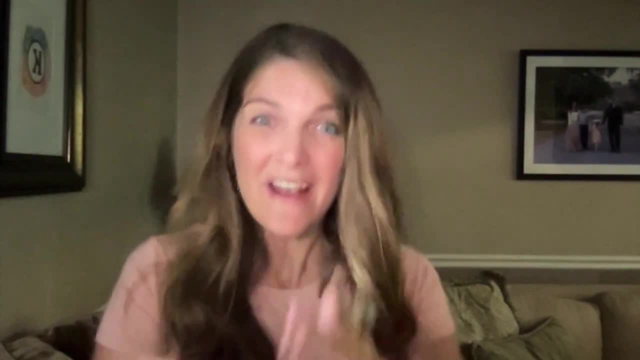 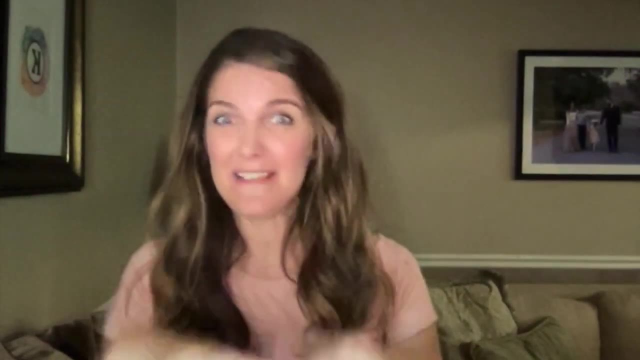 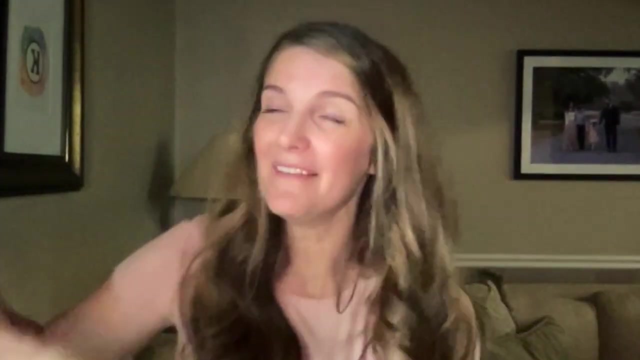 Okay if I don't teach them my expectations. And so on Tuesday I teach them what I want them to do. And so what we do is we go out into the hallway after we do attendance and we practice coming into the classroom, And then we go out in the hallway and we practice coming in And my 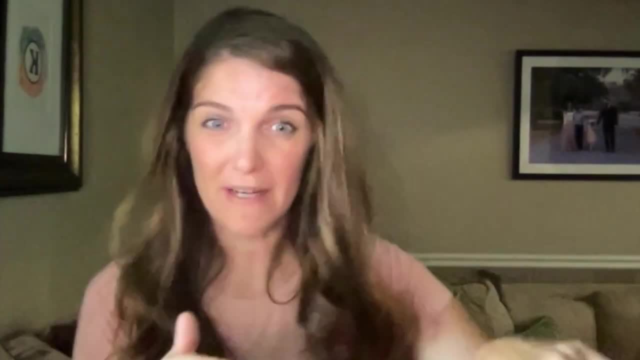 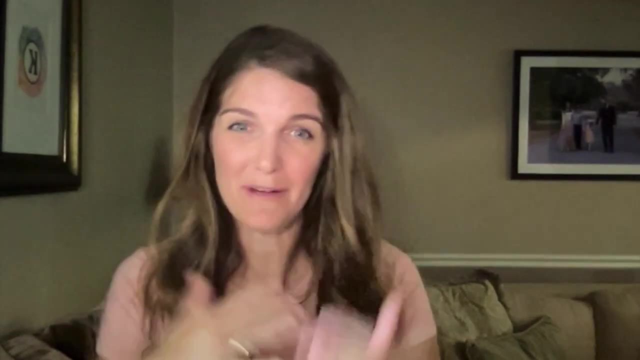 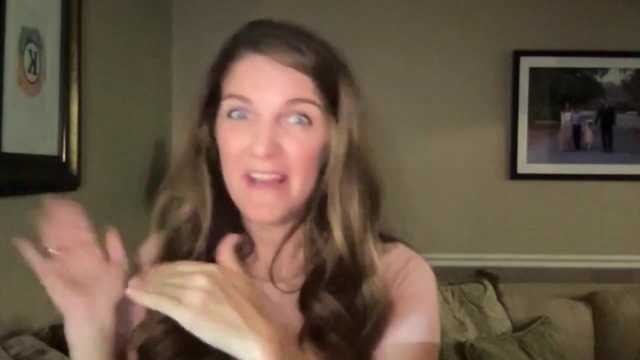 expectation is, when they come into the classroom, they go straight to their seats, they look at the board, they get out everything that they need to in the three minutes timer that I have set, And so we practice that a couple of times because that's a really big one for me, because if they do, 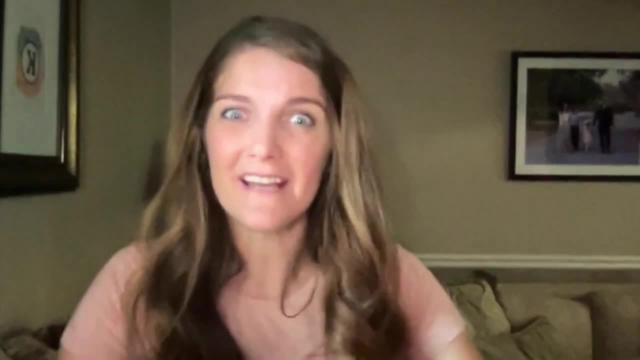 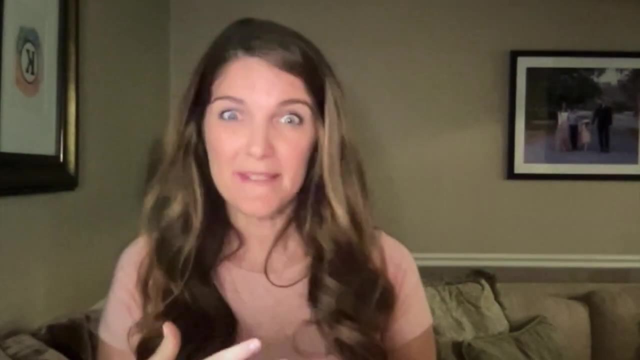 that in the first three minutes of class, then the rest of class, the rest, the next 50 minutes, can flow like that And I don't have to get angry and upset that they're acting crazy when they come into the classroom. So that's Tuesday. I really, really established. 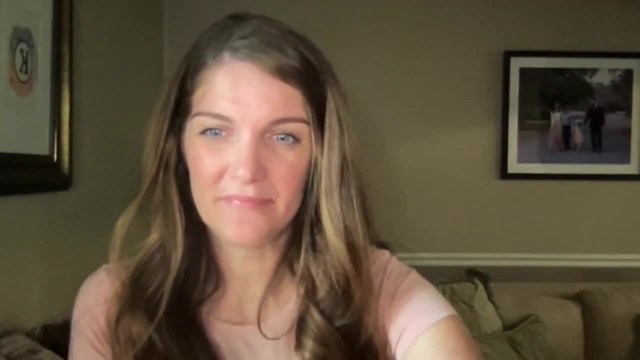 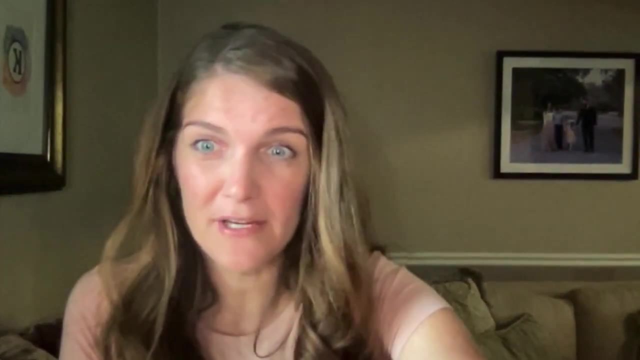 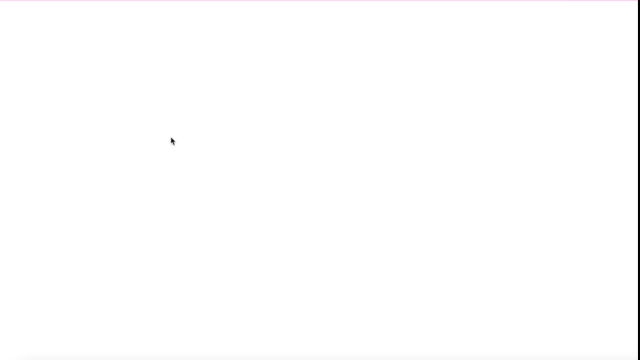 That procedure And then, after that, we have an activity, a building relationships activity, which is a student questionnaire, And let me go ahead and show you what this questionnaire looks like. If you're wondering what I'm clicking here, this is on. all of these resources are available. 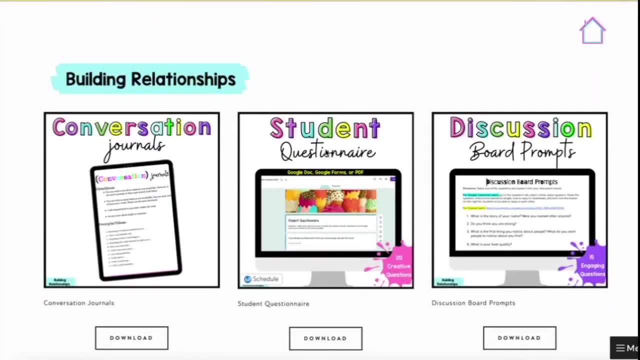 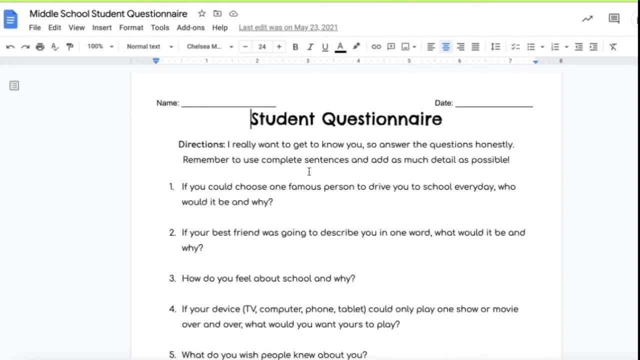 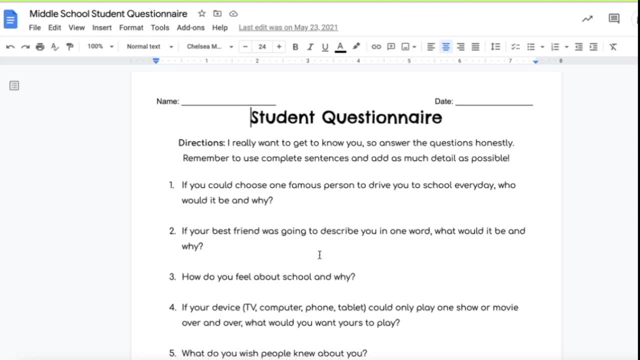 on ELA Unlimited. So this is the student questionnaire. So this is the student questionnaire. It has 20 questions that are beyond your basic questions. It really gets students thinking So, like, how would their best friend describe you? What's some basic question? What do you wish people? 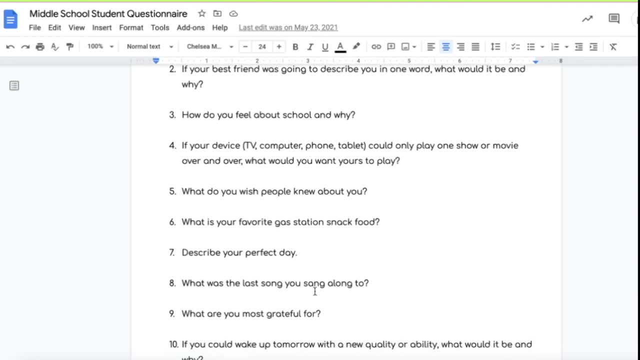 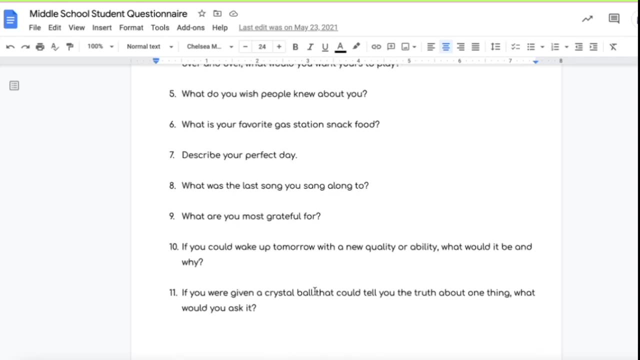 knew about you. And then, what's the last song you sang to? What are you most grateful for? If you could ask the crystal ball, they could tell you one truth about one thing. What would you ask? I love their responses to that question And it just keeps going. I actually have it as a 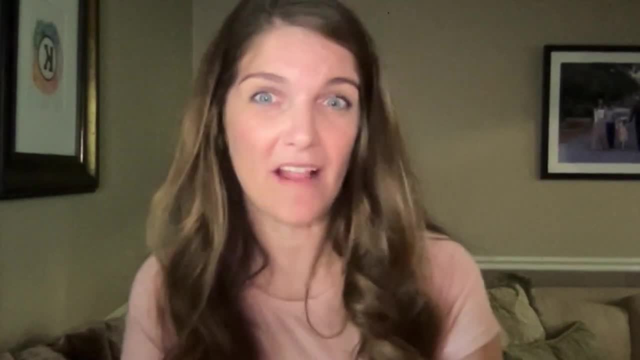 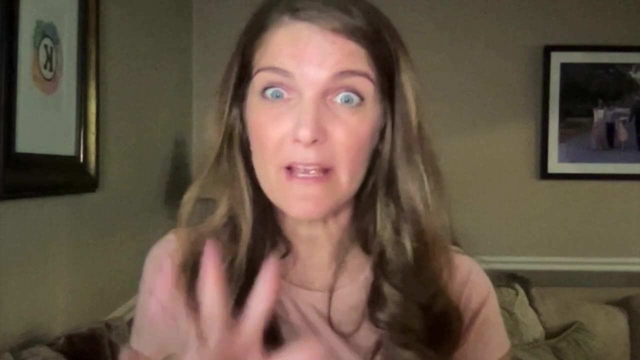 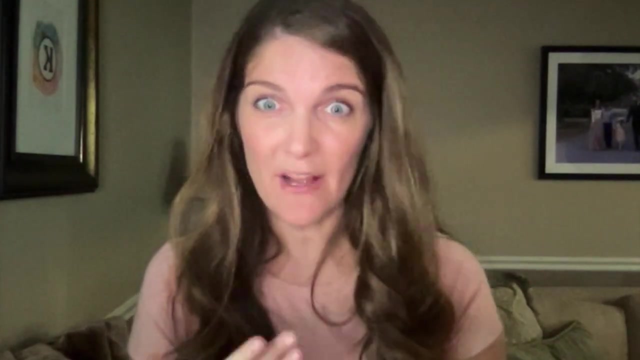 Google form. So hopefully they have their technology by them, But if not, I can print it out And they just take a few minutes of independent time to answer these questions. And what it does is: number one, it tells me about them because I go through and I read them. And number two, it gives me a baseline of 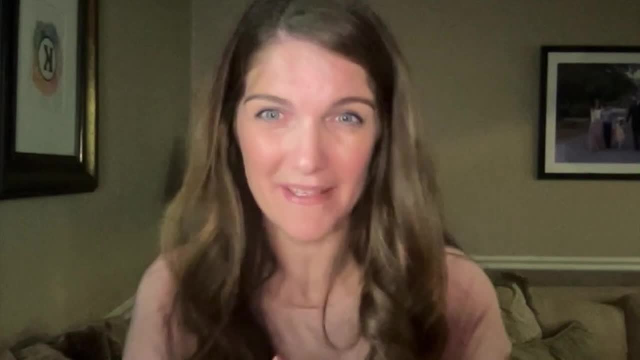 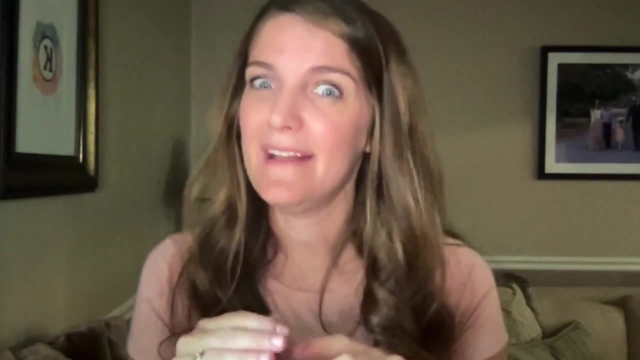 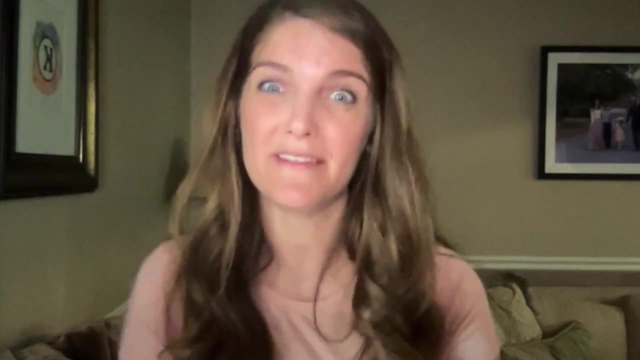 their writing ability, Are they using periods, Are they capitalizing things? Are they writing incomplete sentences? Kind of shows me what we need to work on And, to be honest, the last couple of years I've been surprised at the lack of periods and capitalization and that kind of stuff. So it gives us a good 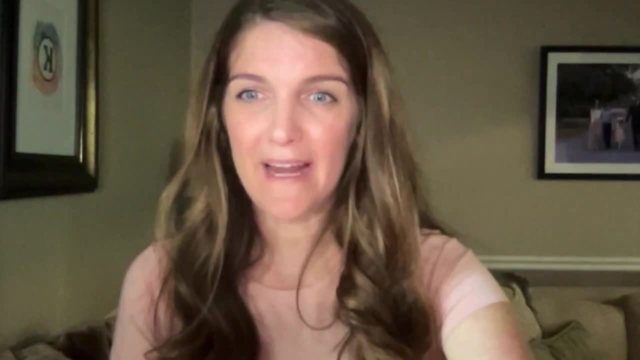 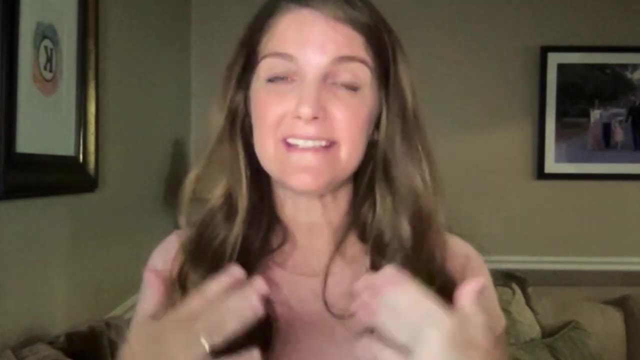 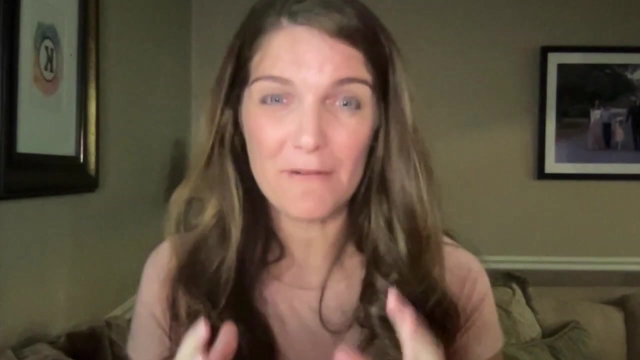 baseline of where to start. After we answered those questions, ask for volunteers of who wants to share their favorite question and answer. Again, it establishes that we share ideas in this classroom. We it's what I call a collaboratory, So we really work together, we share ideas and we. 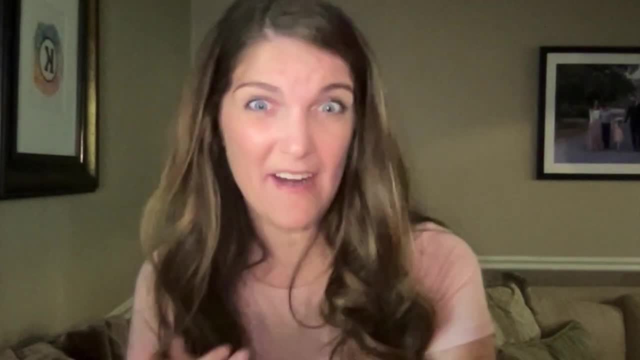 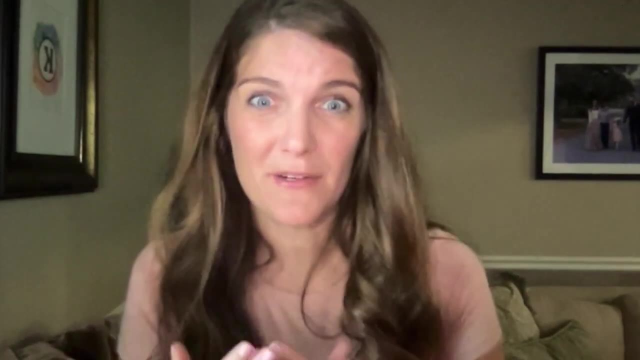 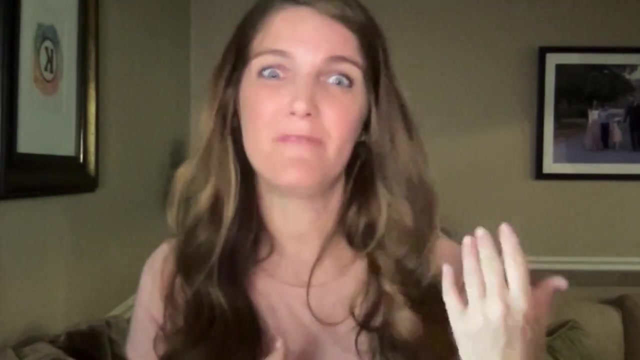 respect our ideas. So before we share, I'm like, okay, who wants to share? We all have different ideas, It's all okay. I really work to create a positive classroom culture where every idea and everybody's point of view is accepted And we may not agree. 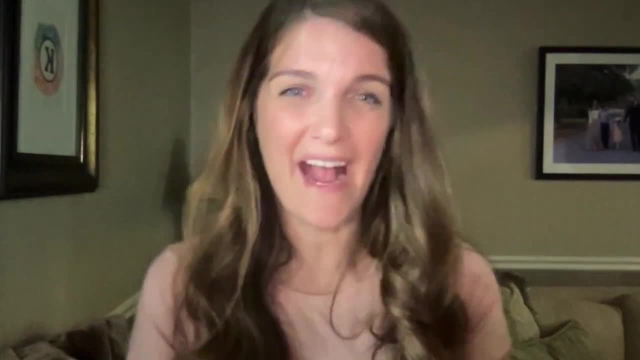 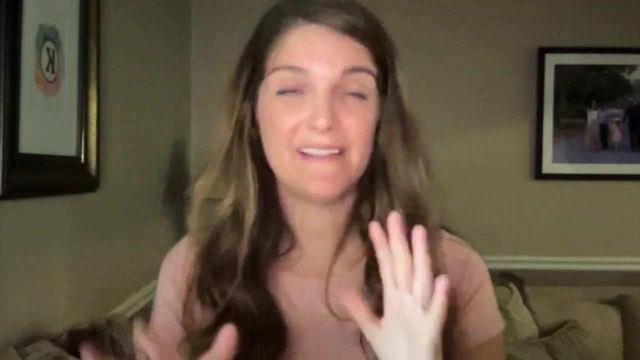 with you And that's okay. We don't have to agree, But we don't have to be mean about disagreeing. Does that make sense? We celebrate the differences. After that, tell them that tomorrow is going to be a really fun day and that we need a water bottle. So we can do a little. you know, we can do a little. 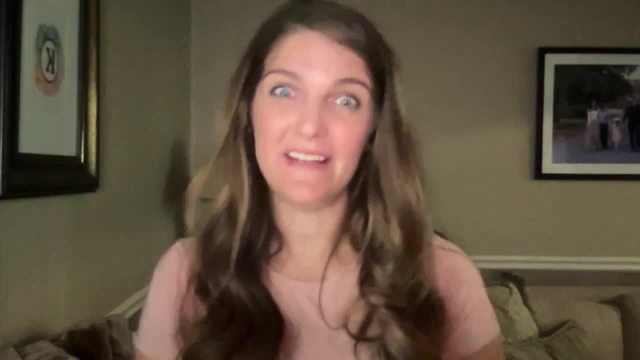 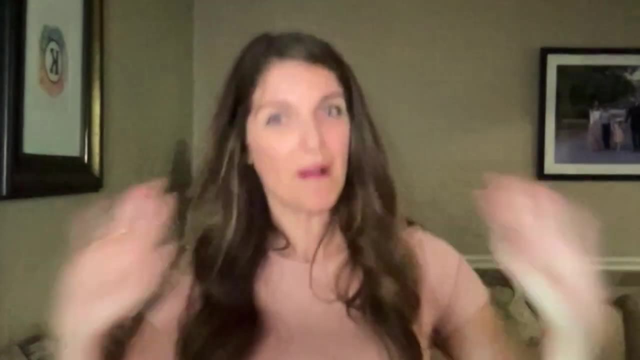 water bottle flipping activity. And not only that. they need their class notebook, because we're going to start learning how to set up our class notebook. So that's the end of day two. You probably need to go home and take a nap. I understand. the start of school is real, It's. 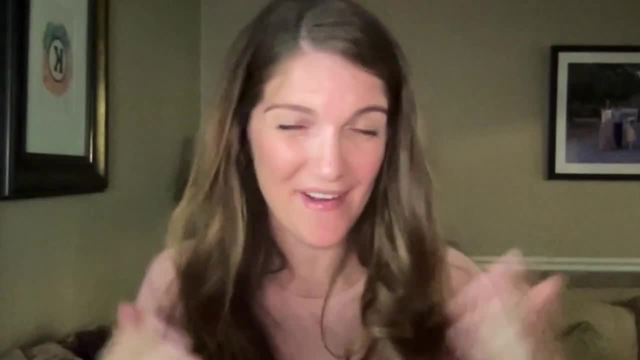 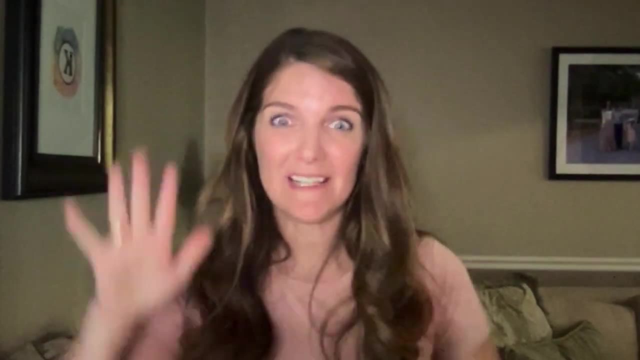 stressful, It's exciting, It's like you're on on on all the time. All right, so here we are. It's Wednesday, We're rested and ready to go. So what I do first is I have my agenda slide. 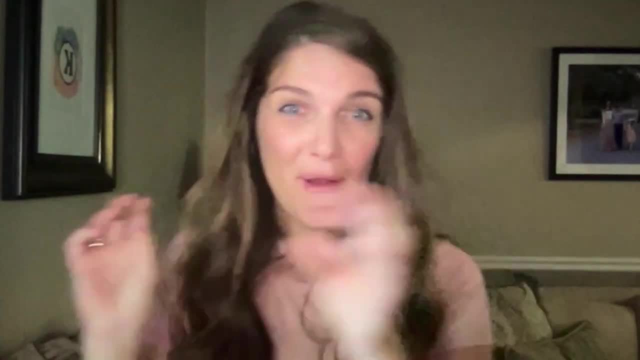 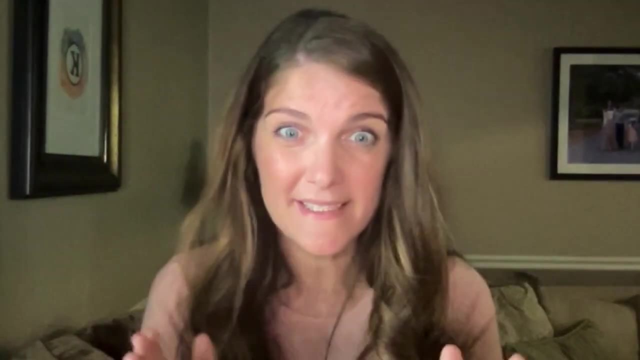 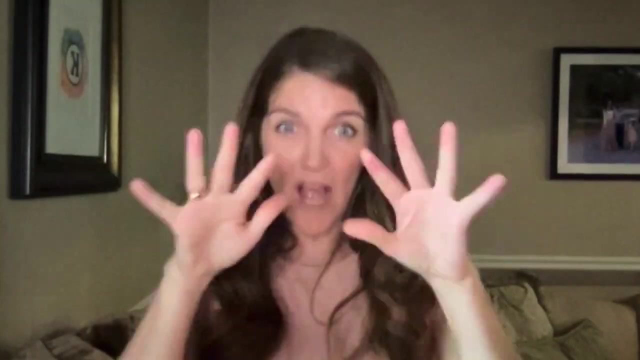 posted on the board and we practice and we see who comes into the classroom correctly, Because we taught that procedure yesterday, So that should be reinforced today. What you need to do is make sure that students are doing that Really, really praise students who come in and get all their 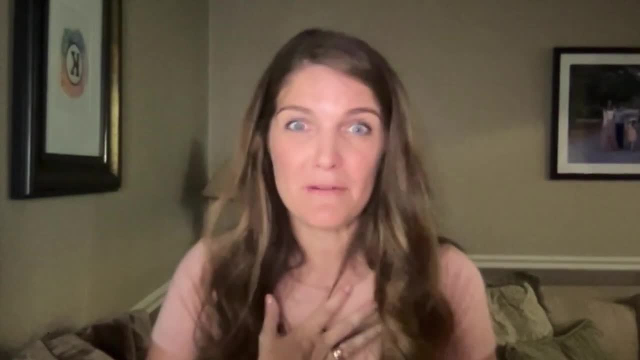 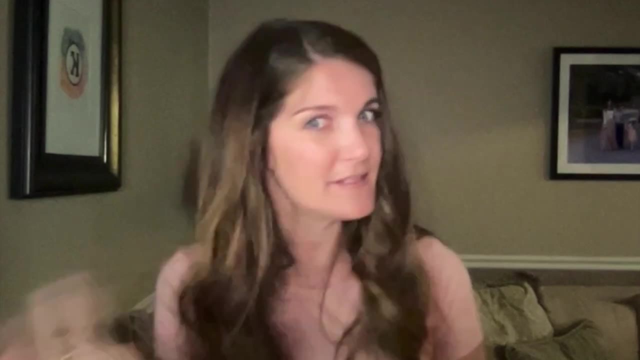 stuff out in the three minutes. I have found as a teacher what really works for me is that I say: if I see someone not doing it, like just staring into space because you'll have that too, if you see someone doing that, look for someone who's doing it correctly And I'll be like, Oh my. 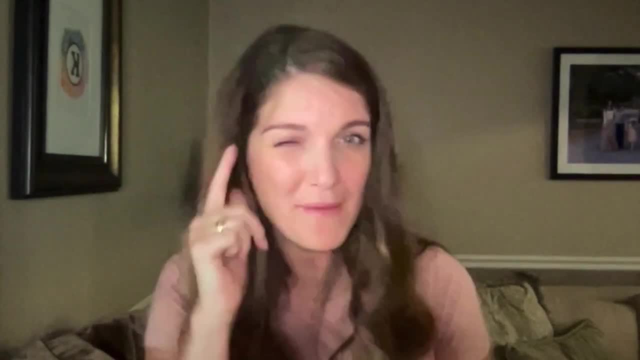 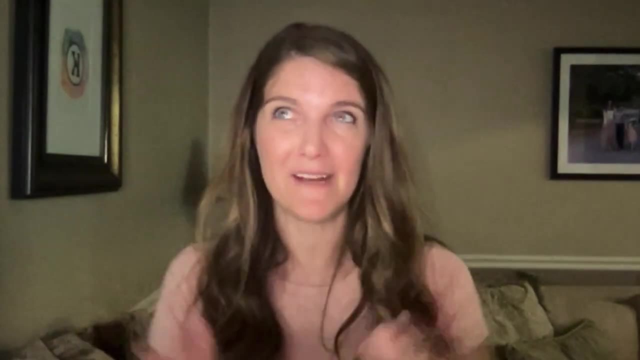 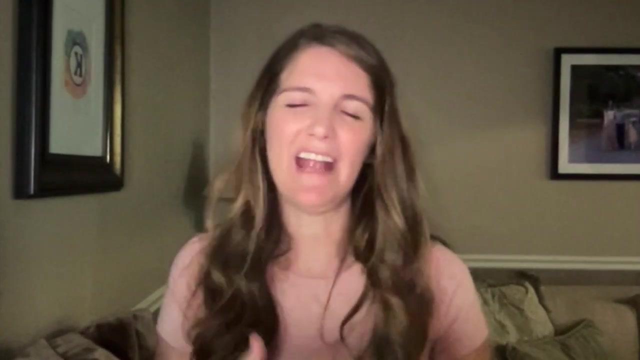 gosh. Jake, thank you so much for remembering what we did yesterday and get it following the instructions, And that really sometimes snaps the people that are just staring in space like, Oh, I have a procedure And so I focus on the ones who are doing it right, And that really, really helps. 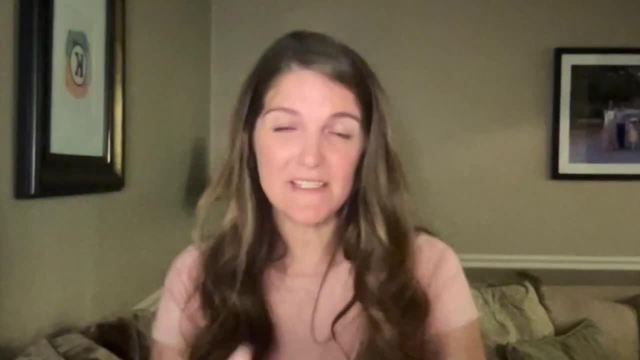 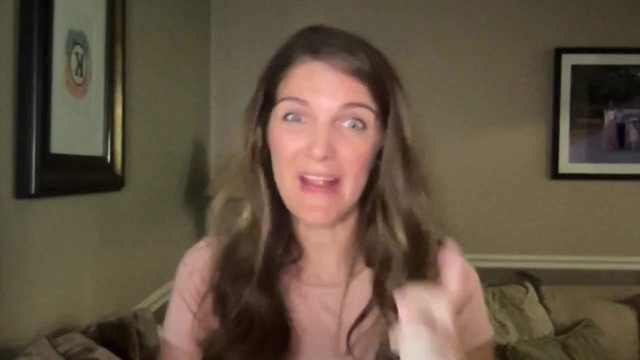 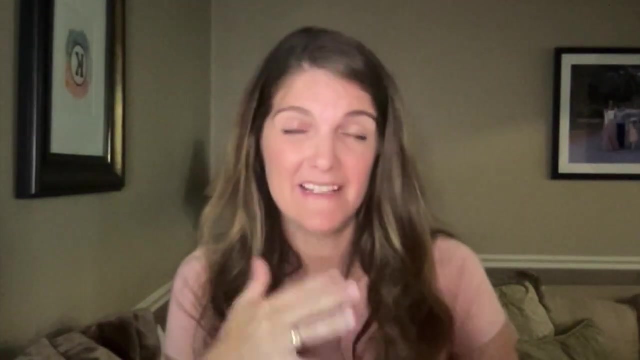 get everybody else on board. So they come in, there's an agenda posted with everything they need for the day And then after that I get over their names one more time, Usually by Wednesday. I'm pretty good. I might struggle with some phonetics like pronunciation, because we have a really diverse 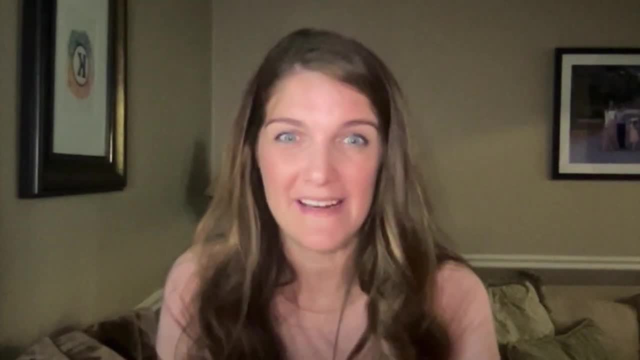 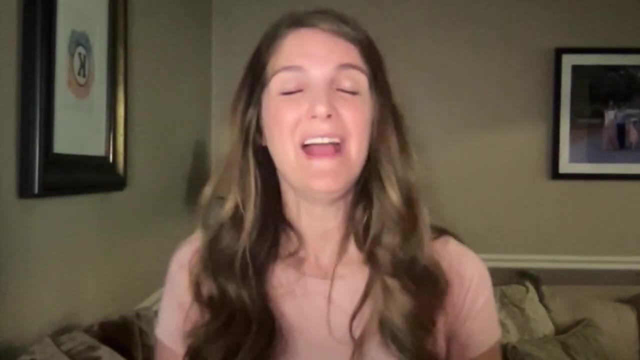 school, which is great. So what I do on my sheets, I make sure I write it out phonetically so I can get their names pronounced correctly. After I do their names, it's time to teach them another procedure, which is how to set up their class notebook. The old school. 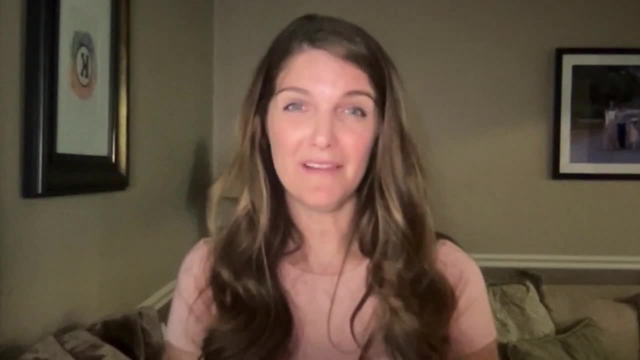 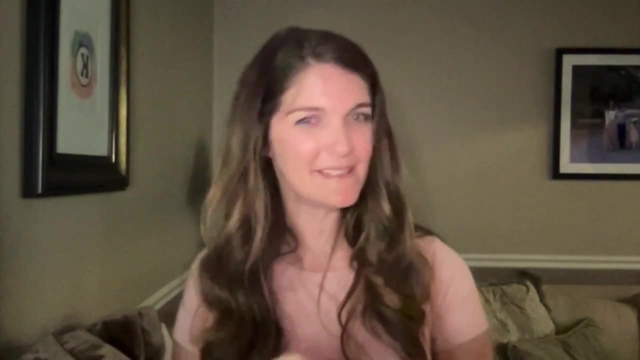 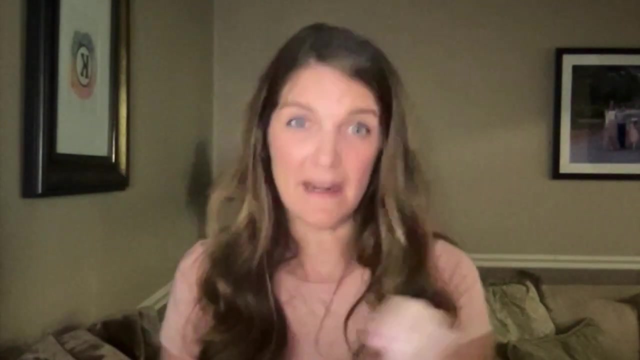 I've been teaching 18 years, but I love a paper notebook. I don't know anybody else with me. Are there any young teachers out there who are like I? like some paper notebooks too? For me it's super. um, it's a great way to keep students organized. I think just the practice of pencil to paper when. 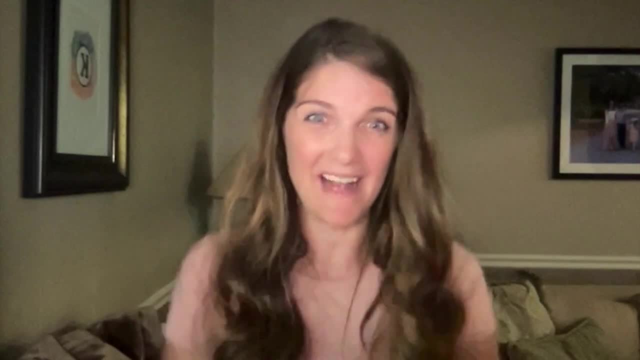 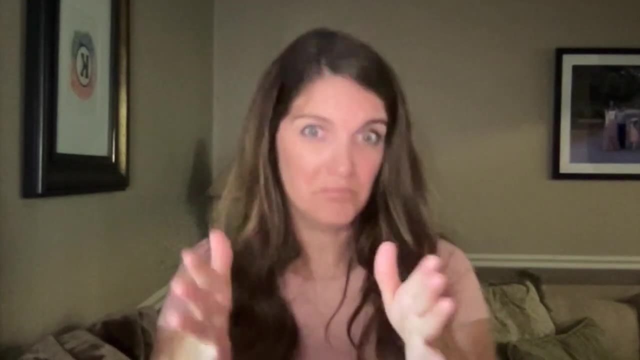 they're reading does something. it makes them like strong connections in their brains. So I love having a paper notebook. I tried a digital notebook one year. It didn't work for me. might work for you, But for me I use a paper notebook. I'm going to link. 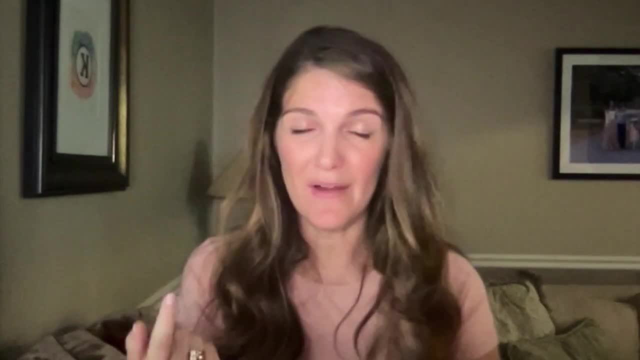 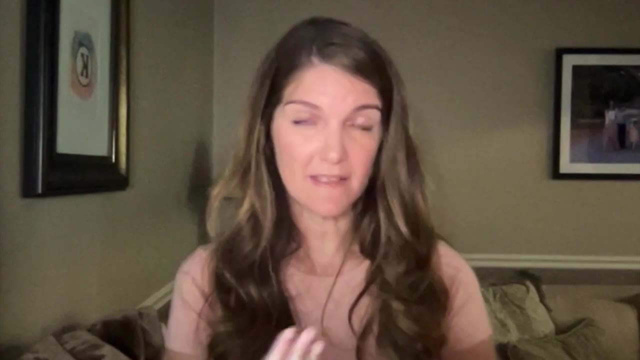 how I set up my class notebook, but that is how I that is. the next procedure that I teach my students is how to set up their class notebook. So when they come into the classroom, they look at their agenda slide, they get out everything they need and then they set up the notebook, which is always. 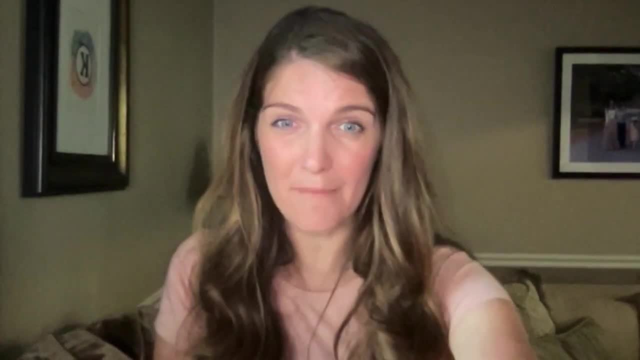 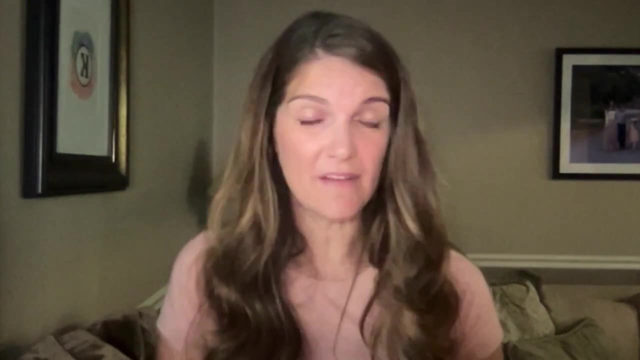 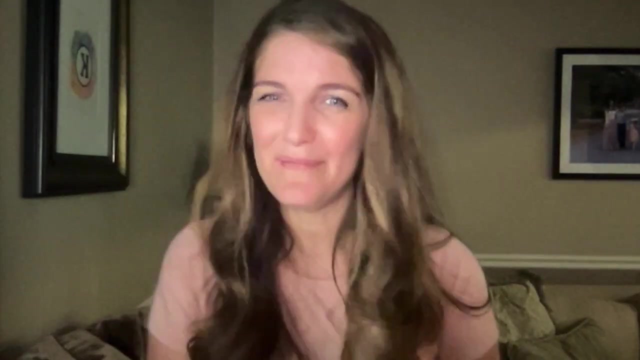 on the back board. So after we go over that procedure, we start our bell ringer activity. So I use bell ringers almost every day In order to get them engaged and started. I pick a really fun- what I think is a fun- bell ringer and I've had some positive feedback from 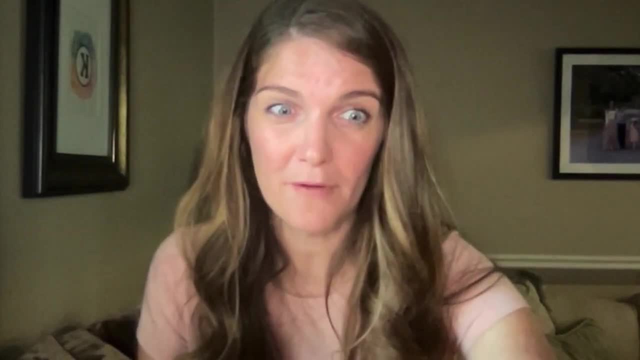 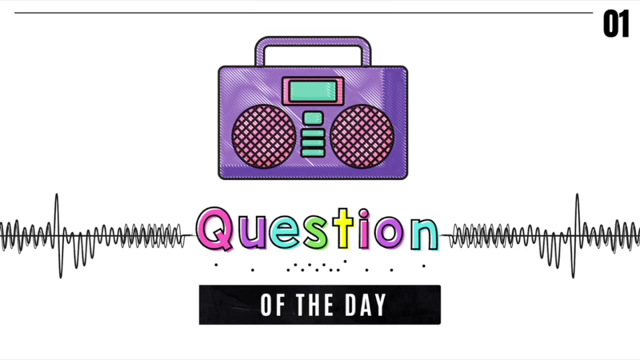 the students about the bell ringers, So let's check out this first bell ringer that I do. So question of the day is all about getting students in the habit of writing and writing without um expect- I don't know if expectation is the right word- writing without stress placed. 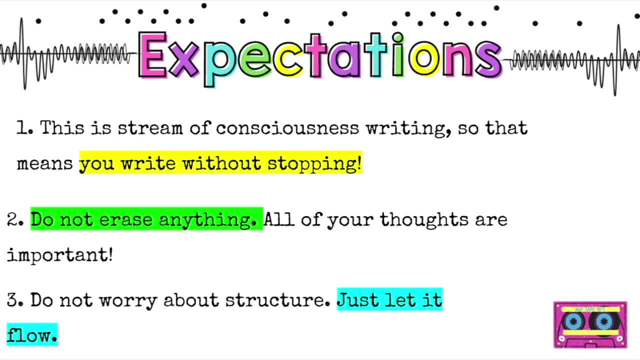 on them, And so there are expectations. It's kind of like a stream of consciousness writing. So I want them to write without stopping. I don't want them to erase anything. I want them to value all of their thoughts and stop trying to censor themselves or like not holding value to what. 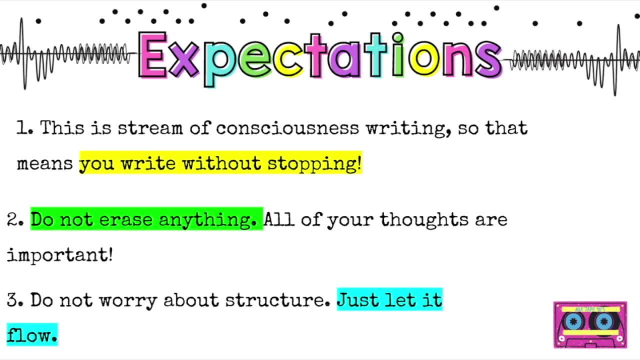 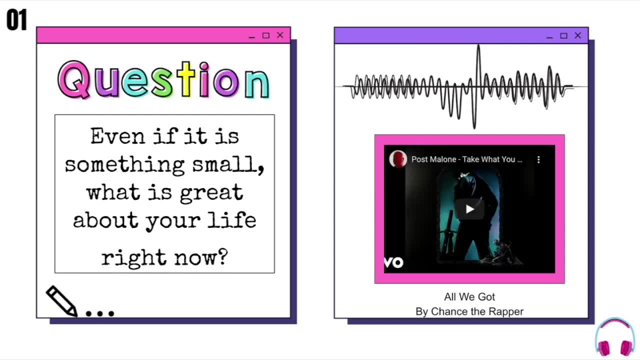 they think, And then I told them not to worry about structure. I just want them to let it flow, And what we do is I pose a question. So this question is, even if it's something small, what is great about your life right now? And I play a song that goes with it, And so, while 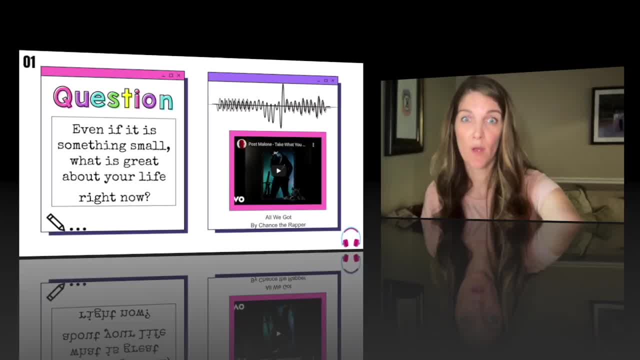 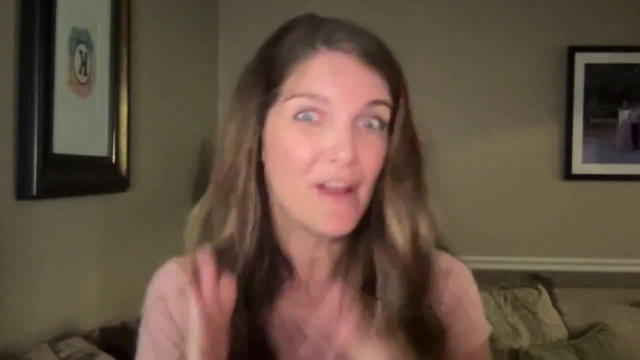 the song is playing, the expectation is that the students are writing, So I try to use a variety of genres for the song. So I tell the students beforehand: this may be your favorite song. You may not have heard this song before, or you may hate the song. whatever, That's cool, You do. 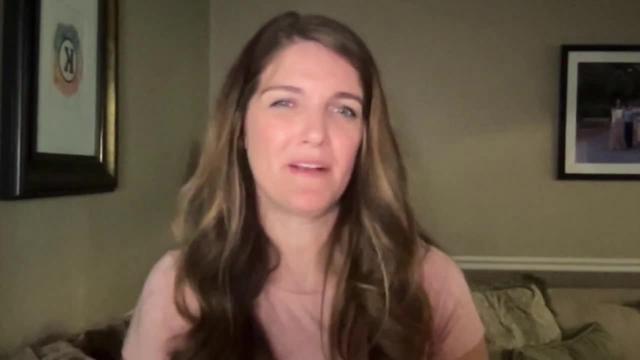 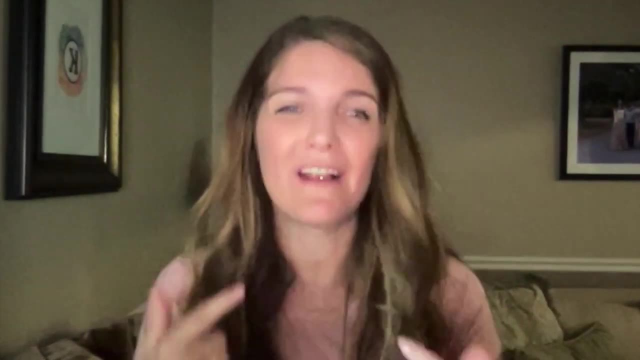 you, but you're going to keep your comments on the inside. And also, what you're going to keep on the inside Is you're singing. That's cool. If you like the song, great, Keep the singing on the inside. that creates a really calm and accepting environment for everybody, Because sometimes in middle school, 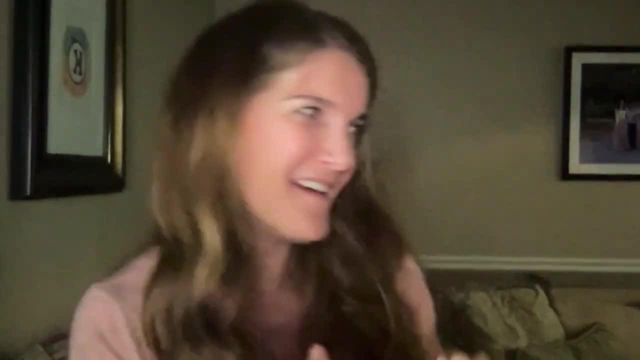 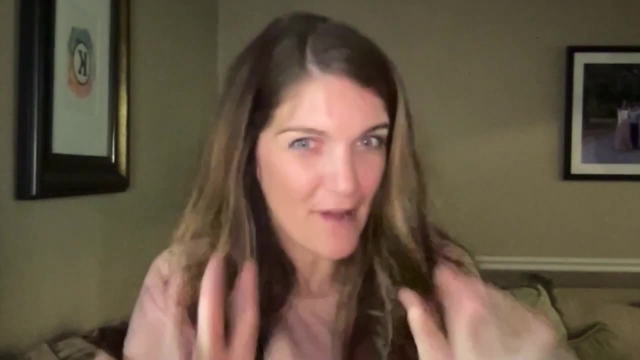 you don't be like, Oh, I love this song. And then you look around and no one else likes it, And so you start to feel self-conscious. So I really set that expectation ahead of time that whenever your feelings on the song, keep them on the inside. It's all good either way And we're just focusing. 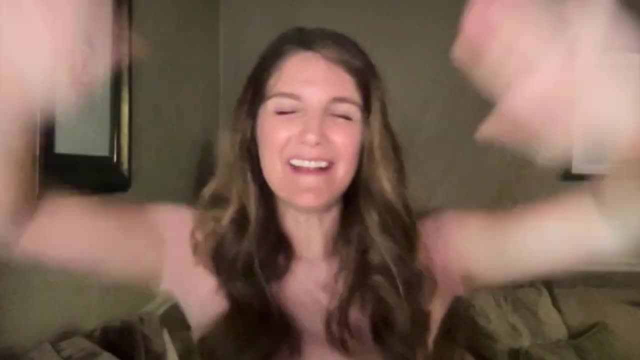 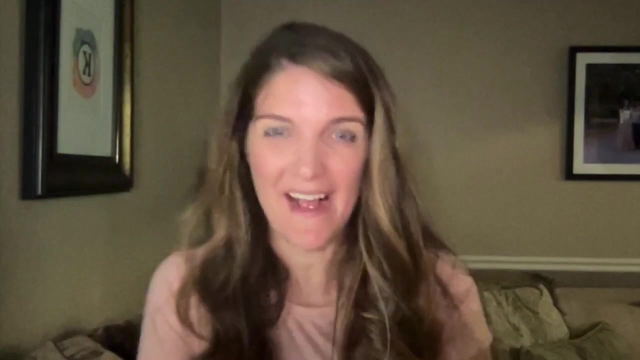 on writing. So that's question of the day, And after that we get to the fun activity of what we call bottle flip, And it's a great fun activity. I'm going to link it below, where I'd have a video or not a video. 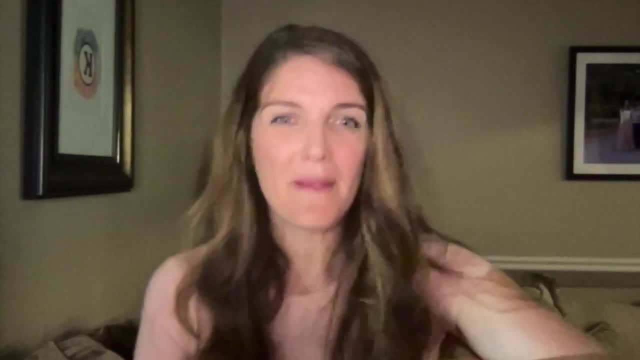 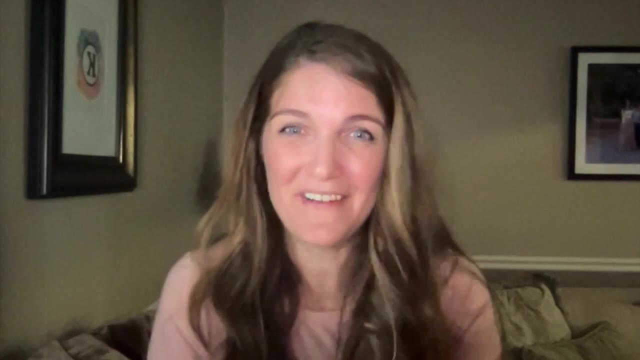 I have an explanation of that activity If you are interested. basically, students flip water bottles. It's a game. It's a getting to know you game. I had so many positive reviews about this game, Teacher saying it's the most engaging thing they've done in their classroom. 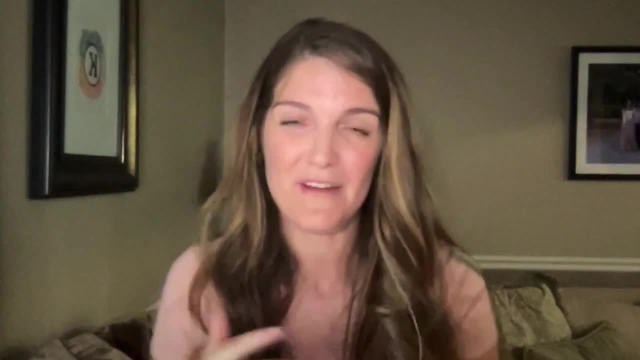 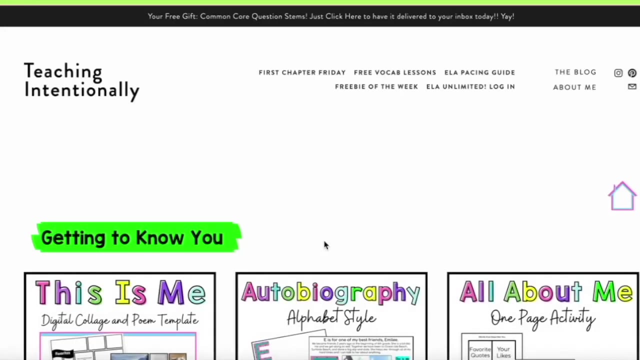 That the students love, So I'm going to link that below if you're interested. It's also available on ELA Unlimited. I'll show you what it looks like If you're an ELA Unlimited person. it's right there. Bottle flip icebreaker activity. 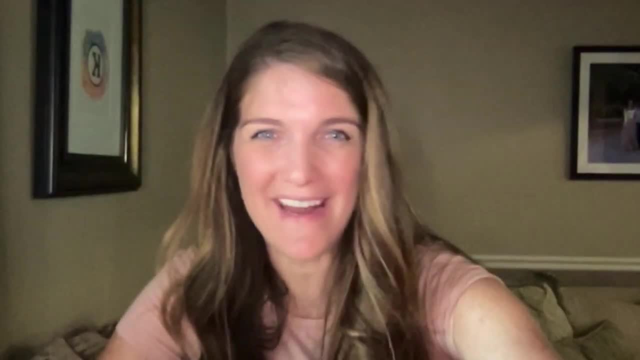 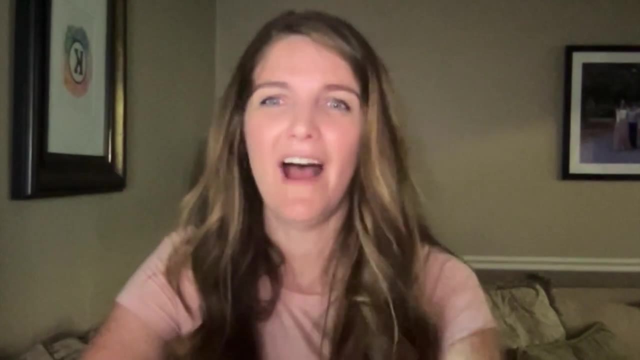 And that is a great, great activity to practice that focus back procedure where you're like, focus up here in five, focus up here in four, And I explained that procedure And I'll show you how to do it. And I'll show you how to do it in the next video. 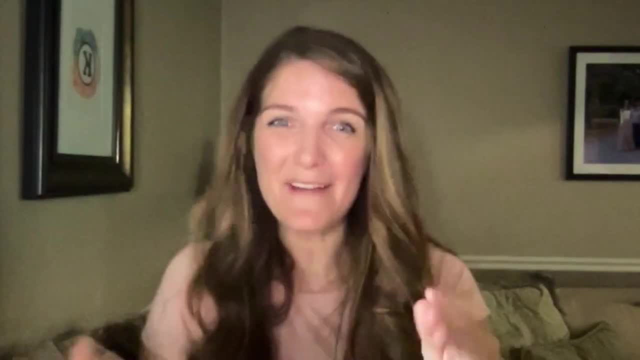 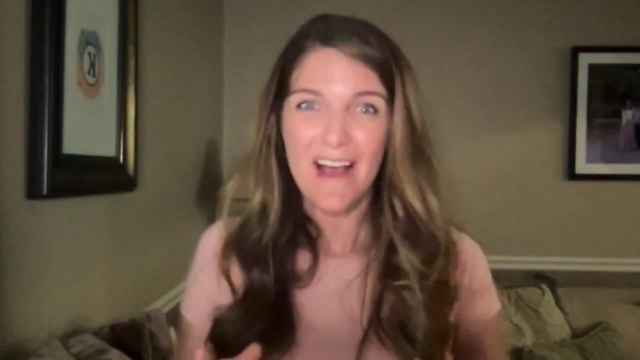 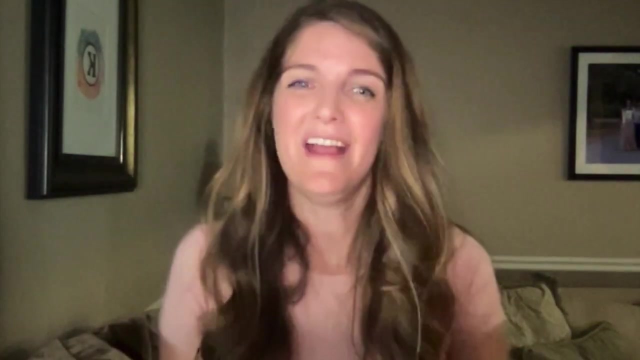 So Wednesday is done by now. You're really establishing some solid routines and procedures for your classroom And you're also setting up a culture of fun, creativity. It's engaging and you're working together, and I love establishing this the first week because students are like 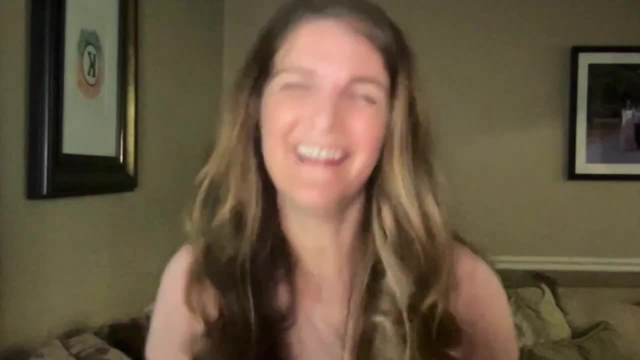 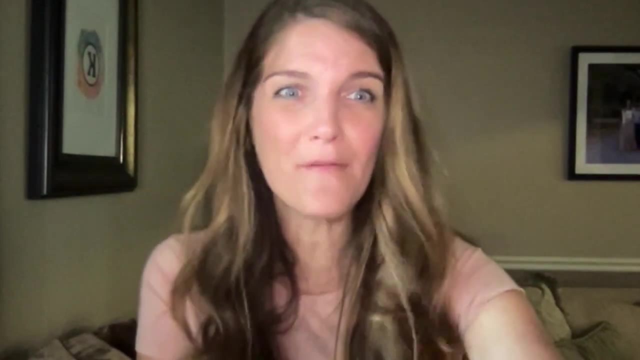 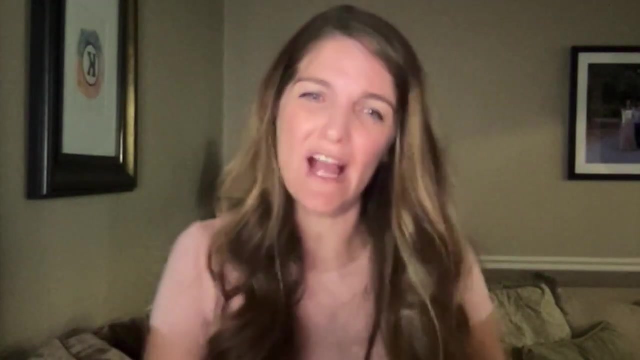 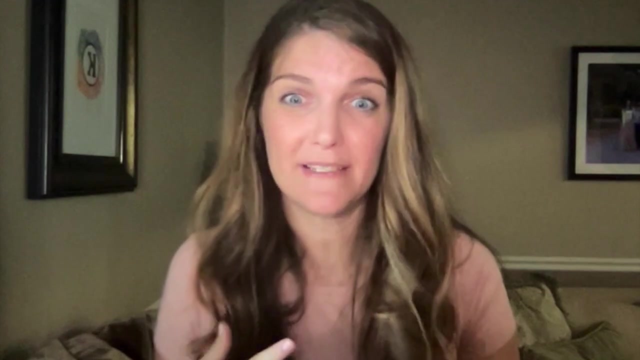 class is so much fun and I'm like, yeah, and it really gets them excited about your subject. and now we move into Thursday. the great thing about Thursday is that we're starting to get into these routines. you're starting to see a flow of things. students like routine and expectations and procedures, because they 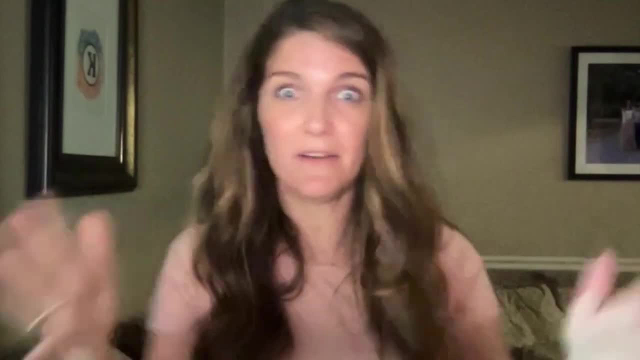 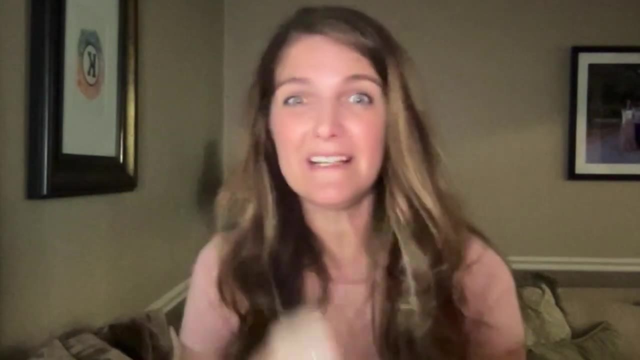 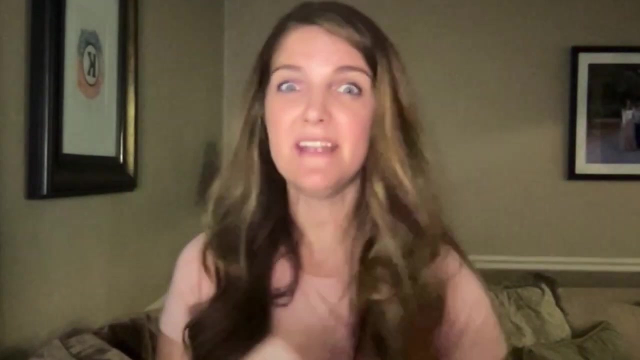 know what to expect every day is not something crazy. they don't just. they come in knowing what to do so you can be more creative. and so Thursday we really start to see things come together. so they come into the classroom like they're supposed, to the agendas posted on the board. they get out what they need. 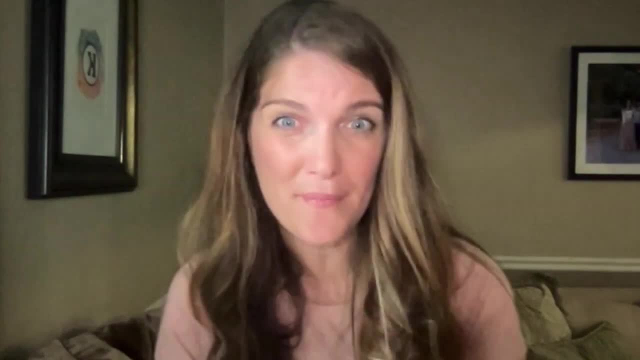 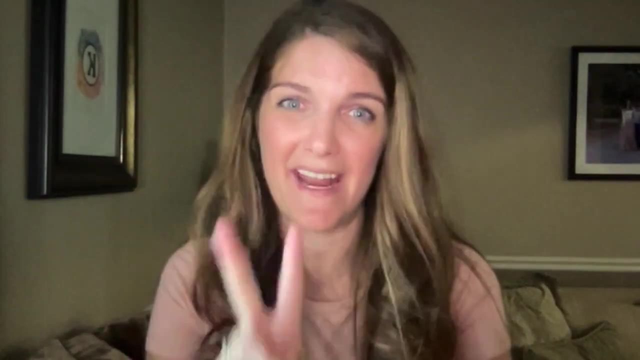 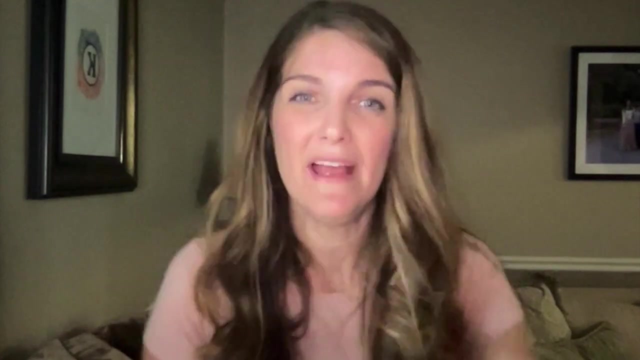 to get out Thursday. we're adding on that. they set up their notebook correctly and then after that we move right into the bell ringer, which is question of the day number two, and then after the bell ringer, we do a getting to know you activity. and now 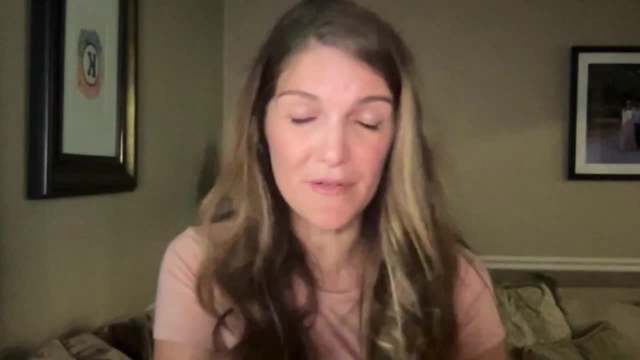 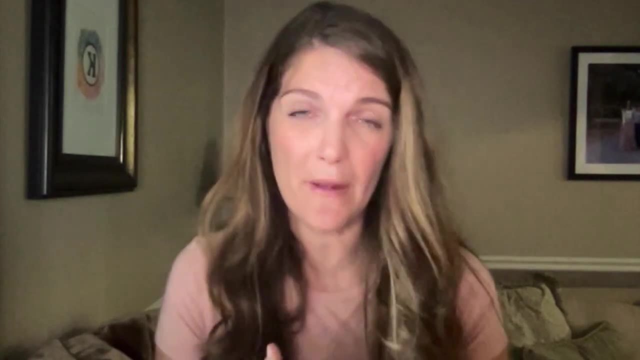 this one is done on the computer. it's a digital collage. again, if you don't have access to technology, or if your students don't have access to technology yet, you can't do it on paper, but I like to do it on the computer, and it is that this is. 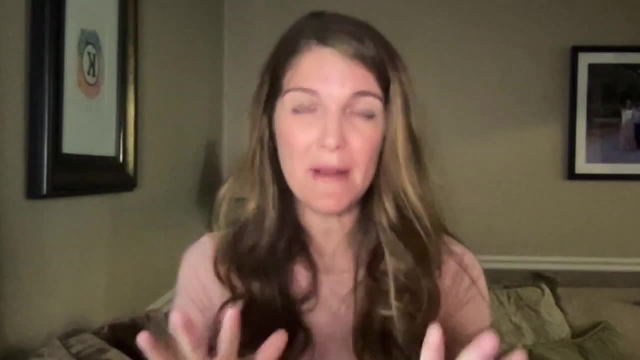 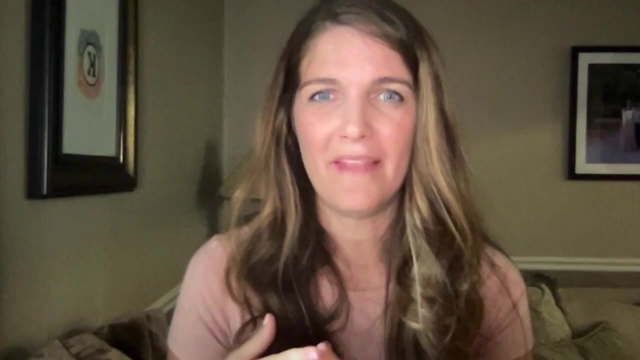 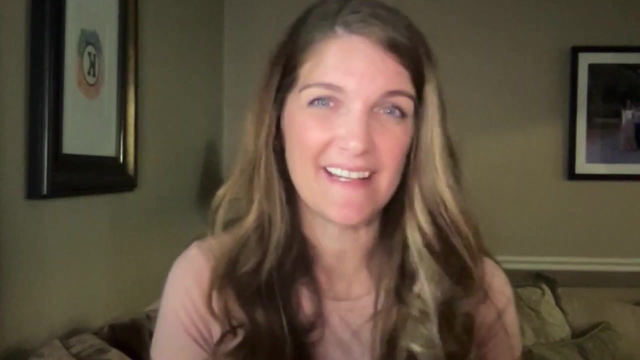 me digital collage. this is an activity where students put in pictures of things that they like to do. so. for example, on Monday I have like running on their coffee. of course, teaching is something I like to do and taking pictures, that kind of thing, so I have images of that and then 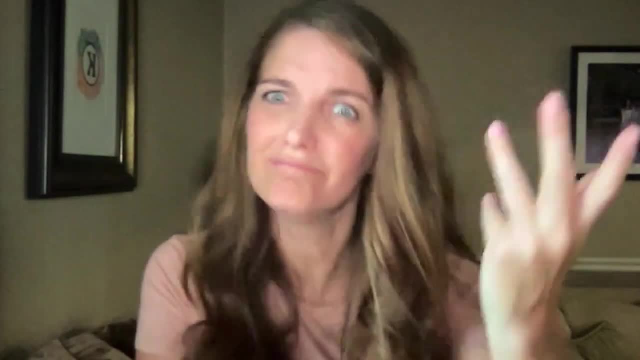 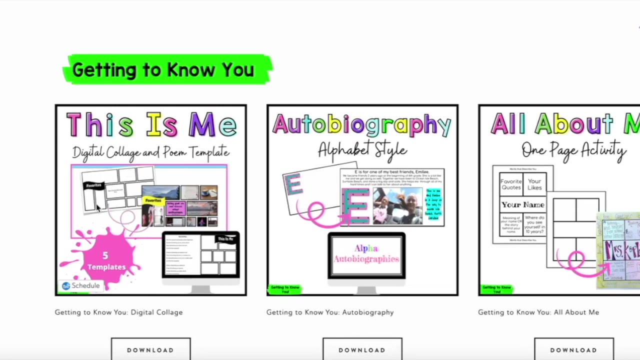 they also have a template to the side. let me just show you this is what it looks like right here. this is me digital collage and poem template. so we have the template they put in their pictures and then, the great thing is, there is this poem where they can fill in the blanks. it starts off with instructions on how to do. 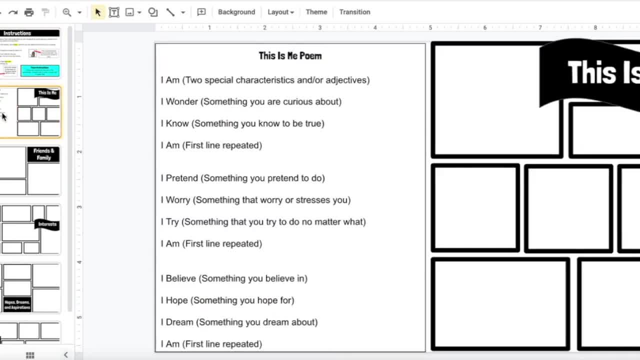 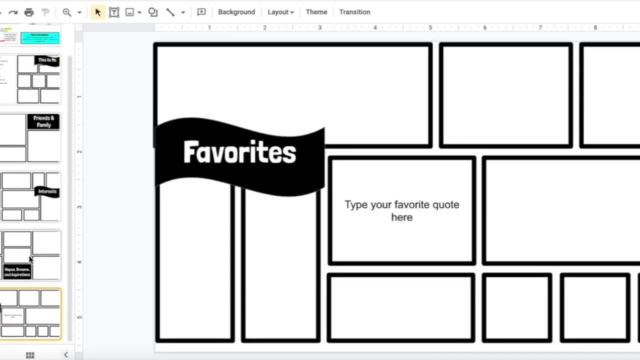 it. and then here's the poem where they put I am and they write two special characteristics about themselves, what they wonder about, and in the parentheses it tells them what to put in the poem. and it's about them. and this resource has different templates that you can do. they don't have to do all of them, because 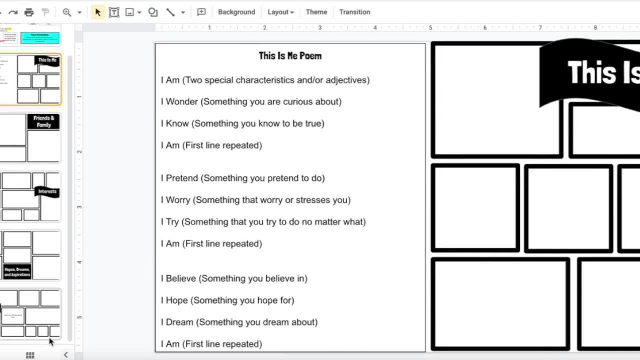 sometimes it can get repetitive. you can just do slide two and then you can put in two and then you can control it, and that's why I like that and the template is really useful anyway, and slide two and three you can choose how you want to do. 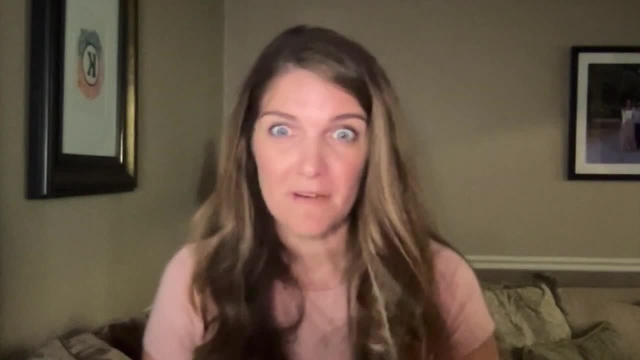 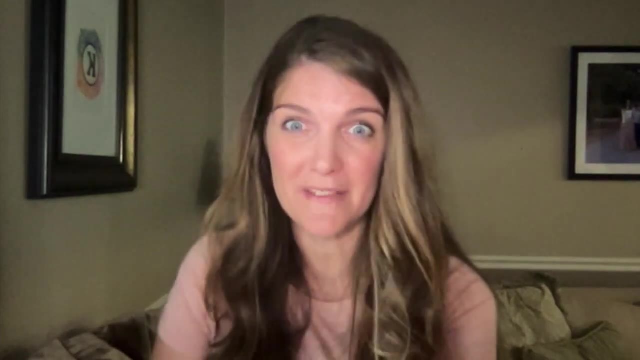 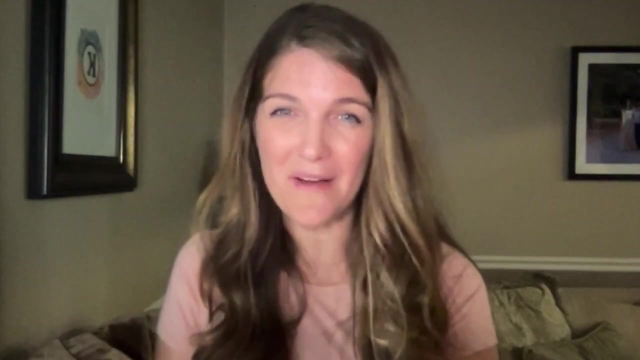 it. so I love students' time to work on this. I circle around, answer any questions, look at their pictures, ask them about it- another good time to start building relationships with your students and getting to know them. and I love this activity because we can print out that first page with the poem and 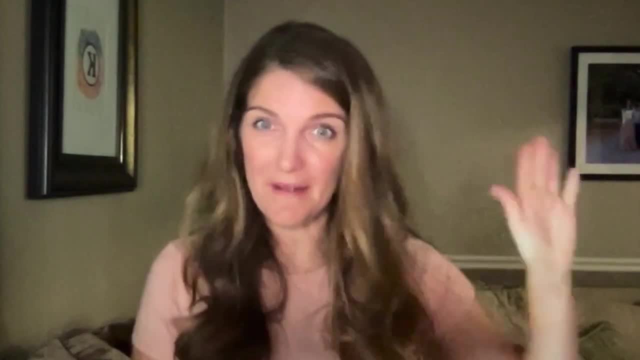 make a really cool classroom bulletin board. in fact I like to put them outside in my classroom above the locker so they can see it coming into the classroom. but if you go to the classroom and you have your own practice classroom and an opportunity for student learning and that's very important. but, like as an 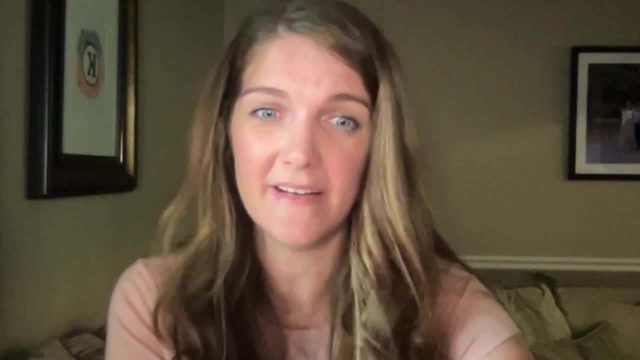 student like a student. if you go to your classroom or a program where you do a job, you just click the link up and it's right on top of your screen or on your desk. so that's the- this is me- digital collage. and that wraps up thursday, and we have one more day. 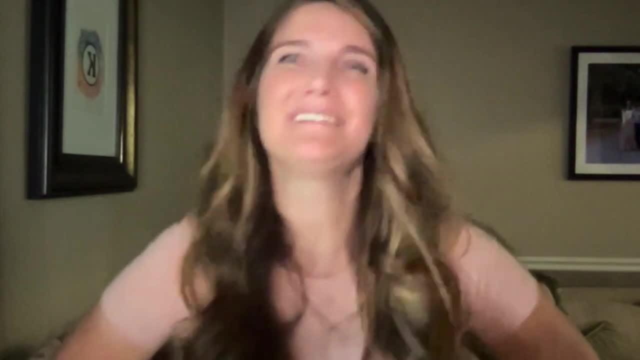 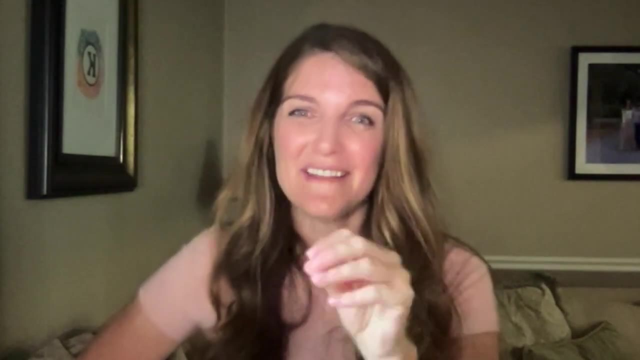 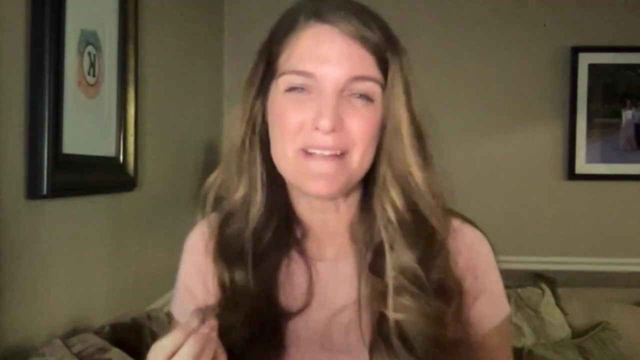 left to go in this first week of school and you are super tired, but you're loving what you're doing because it's systematic and you have a plan. so we're into friday- last day- this is where it all really wraps up and comes together. so students come in, they have the agenda posted. you know all. 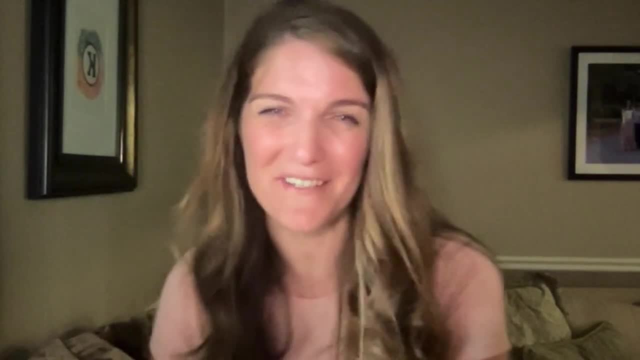 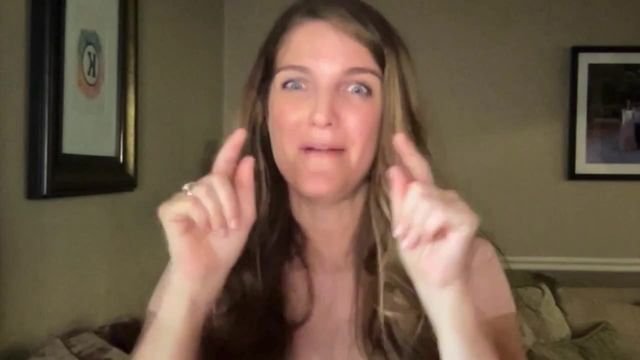 their names because you've been learning them all week. so you greet them at the door with their names. they come in, they get out their stuff in three minutes, they set up their notebook and they are ready to go. and you are praising, praising, praising them for doing exactly what's been.